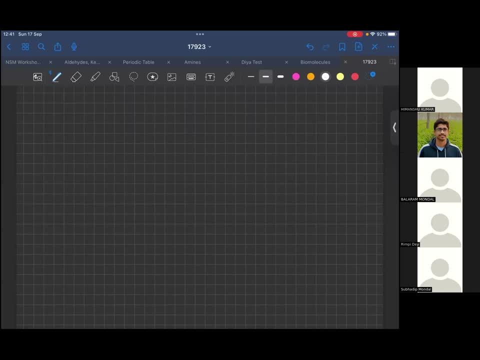 dissipation theorem actually was there. The idea of this theorem was there from the very beginning, like from the very beginning of 1900s, and all but this theorem was actually given by Ryogo Kubo. He was a Japanese physicist and he mainly worked in non-equilibrium. 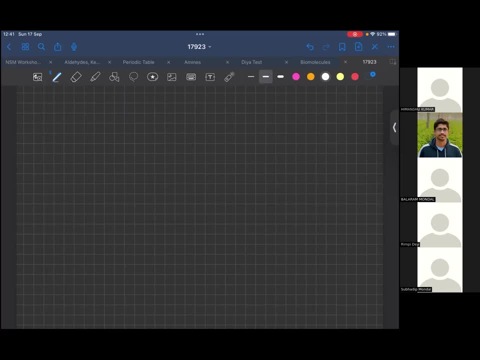 stat, mech and condensed matter physics. So let's start with the term. where does this idea of this fluctuation, dissipation comes? So, firstly, we all know about Brownian particles, right, Like suppose, if we have a container and there is a liquid inside, that. 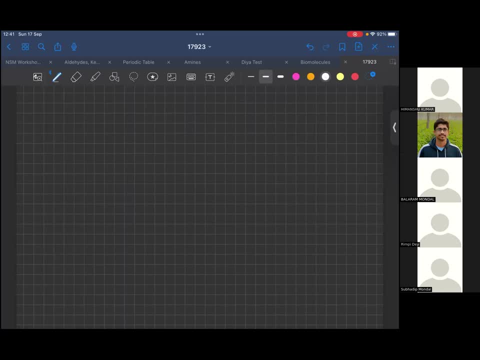 then, and if we tag a particular molecule in there, then suppose there's a container and there are liquid molecules in there and suppose we're tagging a particular molecule, then we know that the motion of this molecule is going to get influenced by its surrounding molecules. So the effect of the surrounding 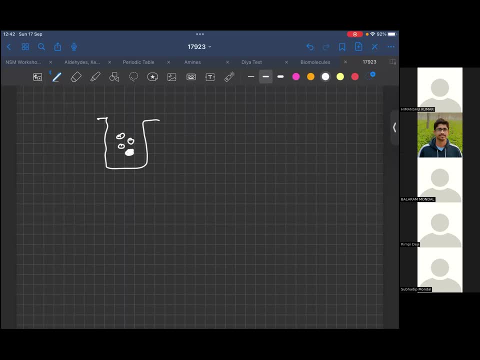 molecules on the particle of our interest is actually given by two forces: one that we call the systematic part of the force- Sorry for the handwriting. So the force is actually given by two forces, One that we call the systematic part of the force, So 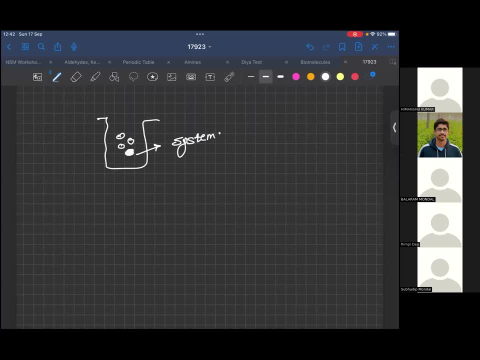 the time and another is random part. So suppose we apply some external fields in our system, Then our normal observation will be that the particles will get arranged here and we'll get our response because of the external force that we have applied in our system. now, this external disturbance, 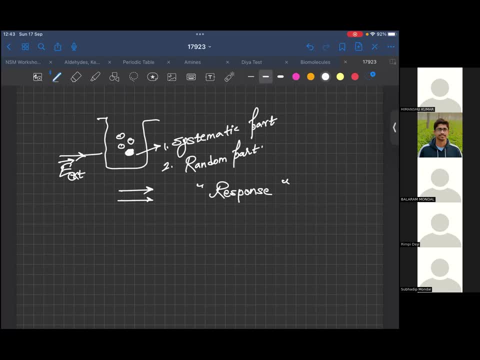 that we are giving from outside and the internal situation of this. yeah, if the particles are neutral particles, then how? the external electric field? and yeah, yeah, considering the brownian particle is a charged system, charged particles, yeah, so so yeah, as i was discussing, so if you are applying this external disturbance in the system, then 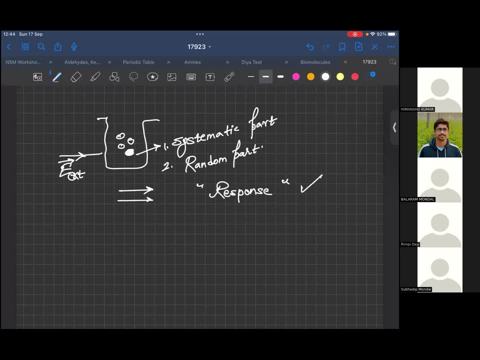 in presence of this external disturbance, there is going to be a response, and in absence of this external disturbance, there is going to be some internal fluctuations in the system. so you have to substitute for the internal dramatically. Now the main idea of this fluctuation: dissipation. 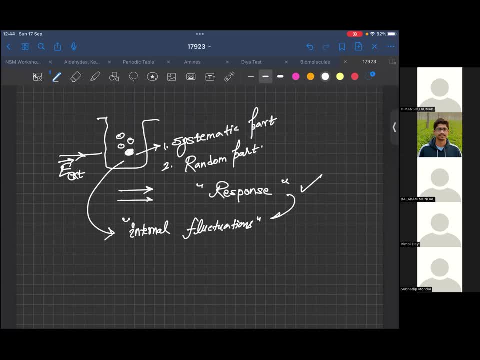 theorem is getting a relationship between this internal fluctuations and the external response. so this basic or not basic, but this idea can be philosophically connected to our own lives, like whenever, if we say we're, you know, whenever we are in working, or if, whenever we are in work, or if we're in family, or your sexual 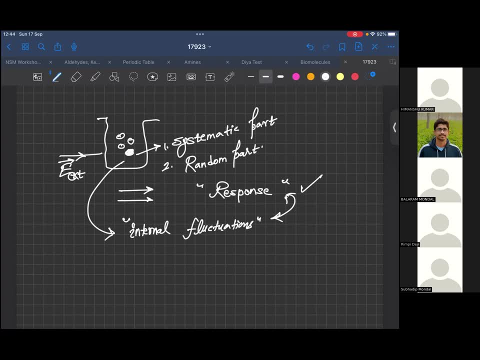 environment. this certain task is the fashioned, who becomes the person who has to react, or perhaps the young when the time comes, or, and it's not charged, and they, they end up in conjecture, and then it becomes extremely difficult. that happens because it reached very high marks on the 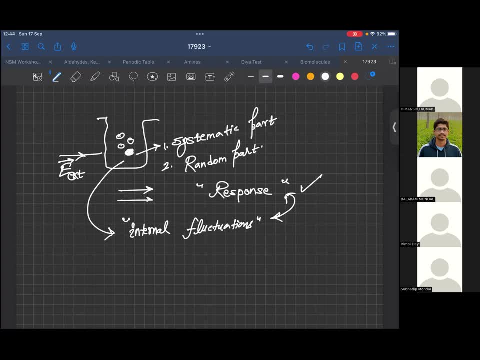 like we were in school or colleges. we were having some fixed time schedule, that we had to go to our classes at time and do things. but if we think about it in adult life and there is no restrictions in us, then that discipline is somehow lost. so irrespective of that discipline, we know that. 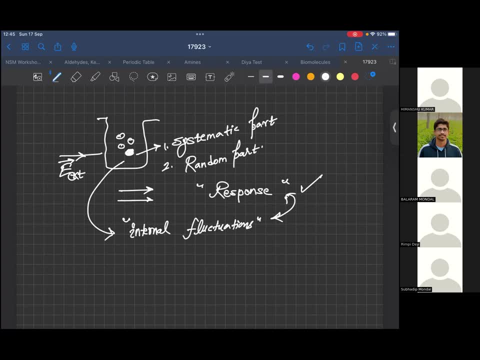 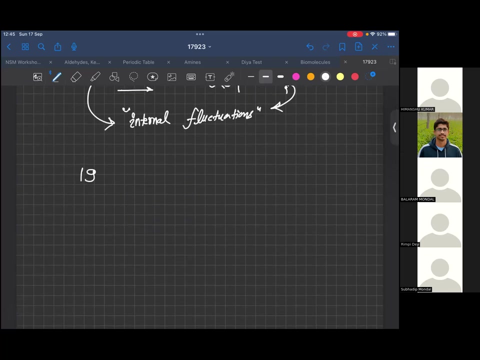 we are working right. so it's like kind of our internal fluctuations and in absence of this discipline, can also lead us to the destination where we want to go. so in the year 1905, einstein uh gave this diffusion constant equation of a particle where he said that diffusion of any molecule 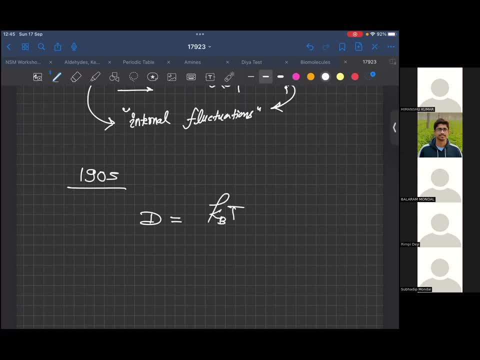 is related to kbt by m gamma. so we know this kbt is the thermal energy of a molecule in equilibrium and this m gamma is our frictional constant. so, like so redox, our entire made of� this one suppose there was, ah, If you or or someone or whistle there. 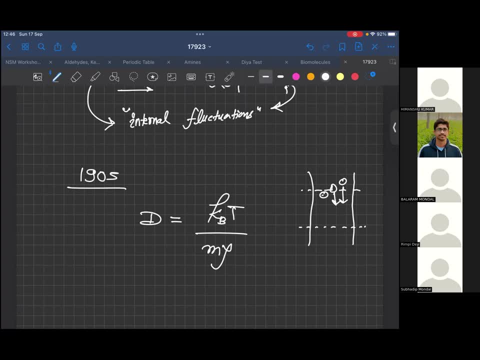 Know there was a do for Lakeway Molecules601.. No, No applied a potential in this part of this tube where this potential is not equals to zero. and now this: in presence of this potential, this liquid molecules are going to drift. 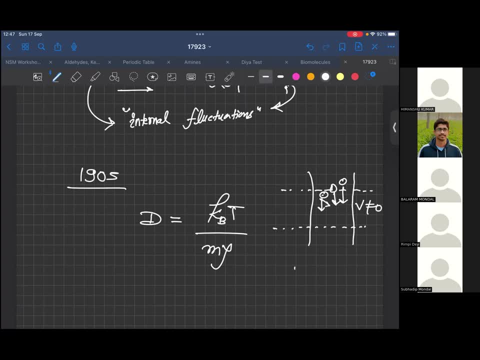 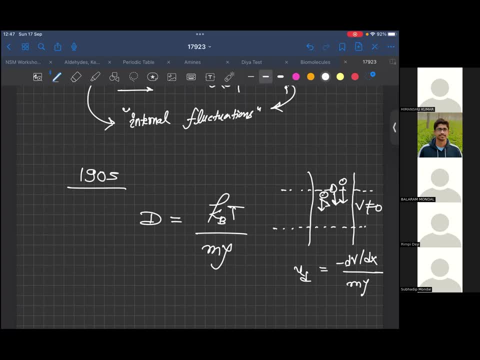 also, there has to be some gradient to move for our molecules to diffuse from one part to another. Now, this non-uniform diffusion process, Einstein, assume that addition processes is a nun sir. so, Einstein, I do that Diffusion processes are definitely going to happen. 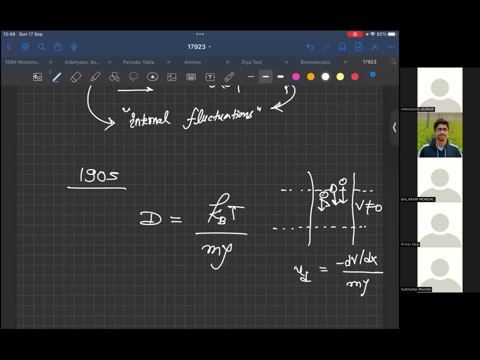 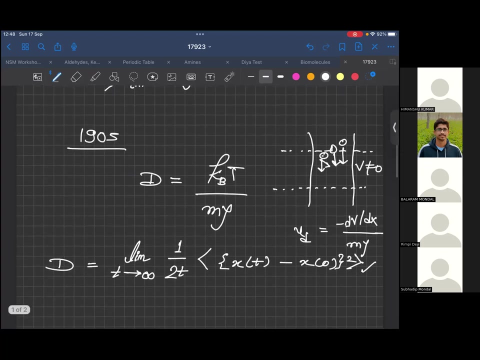 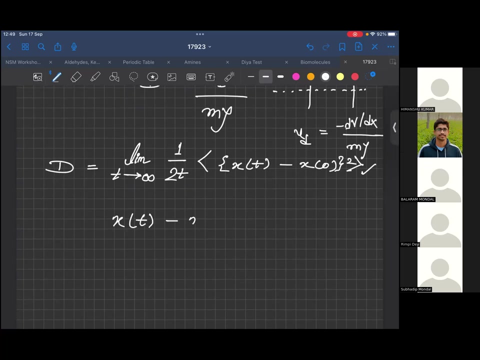 in non-uniform solution. So from that assumption, give a relation that at infinite time things are going to get at thermal equilibrium and the diffusion coefficient will be given by this following expression that I wrote right now: Now we know that position of a particle at xt minus x0 can be given as its velocity and 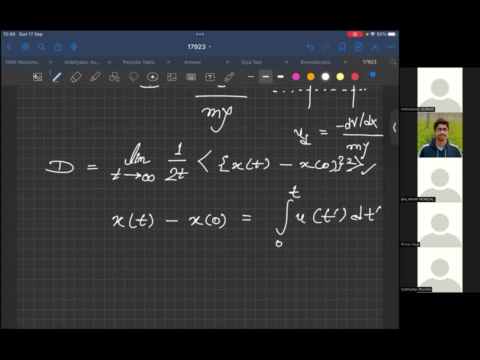 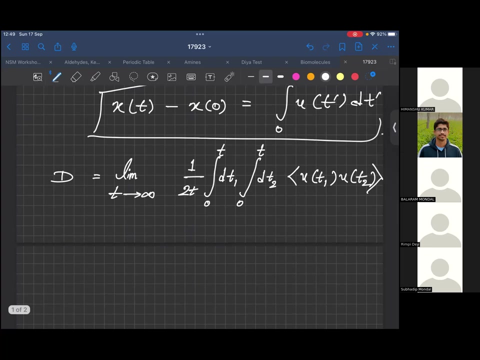 time over time. Now, if we put this expression in the above diffusion equation, then we can see it. So we can see that the velocity at xt minus x0 is equal to the velocity at xt minus x0 is equal to. the velocity at xt minus x0 is equal to the velocity at xt minus x0.. Now 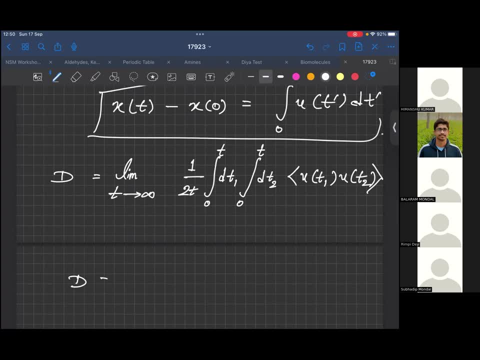 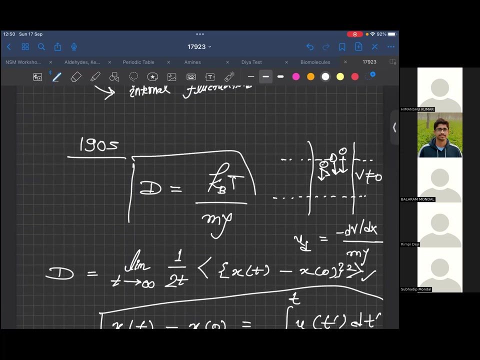 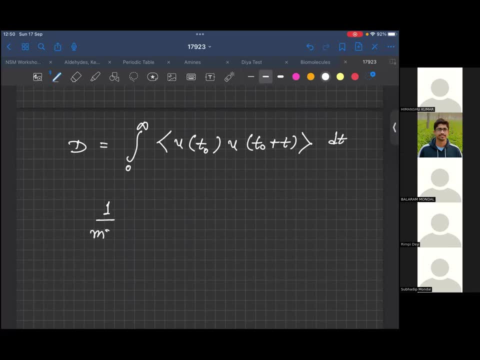 you can write, you can write at all At all, to D by cavity and just putting a value of this D here. So this is our mu, which is not the dipole moment, but the mobility which is the inverse of frictional constant and it is related to the fluctuation of velocity of the Brownian. 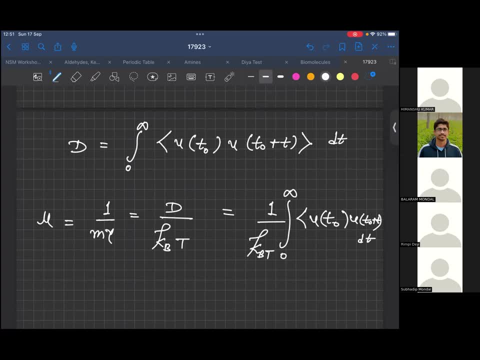 motion and this whole relation, mu is equals to this velocity correlation of this Brownian motion particle. that's underway, That was, this Brownian motion was manifested by Einstein in the year 1905, and hence we know that the idea of the fluctuation dissipation theorem was there from the very beginning. 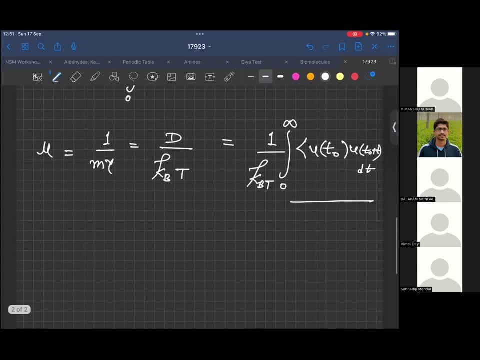 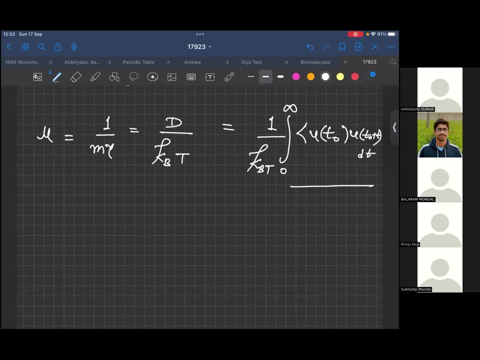 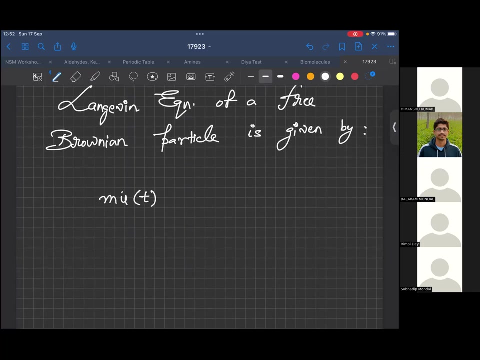 and it actually came into action when we consider the Langevin classical equation of Langevin and the random force. So the most simplest example of a free Brownian particle, the Langevin equation of a free Brownian particle. Now here you can see. this is our frictional part that we discussed from also the Einstein's. 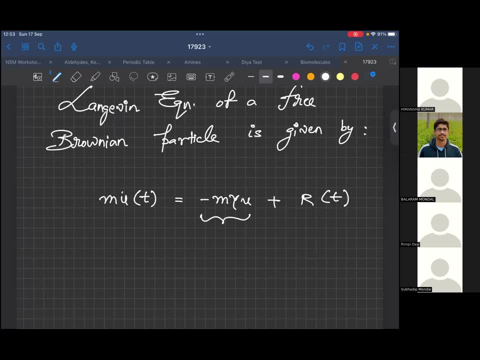 ideology of Brownian particle or Brownian motion. and this part is our random force. So this term is due to the random collision of the surrounding molecules that is having some effect on our Brownian particle. Now for simplicity. and for simplicity, basically, there were two conditions that were assumed. 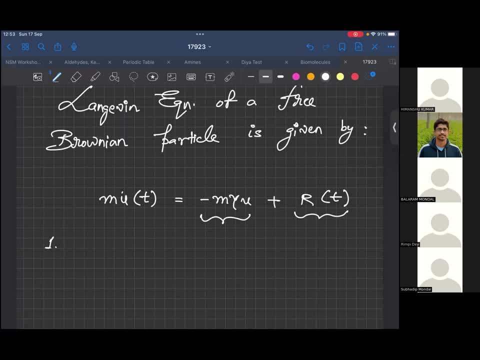 that this RT is Gaussian and the correlation time is very short, like 0.15, 0.12, 0.015.. So it's a fraction of the time that we're actually going to be looking at the random force. So I'm going to go ahead and do a little bit of a zoom in to see if I can get the 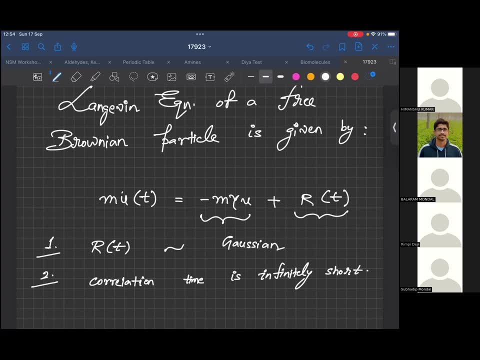 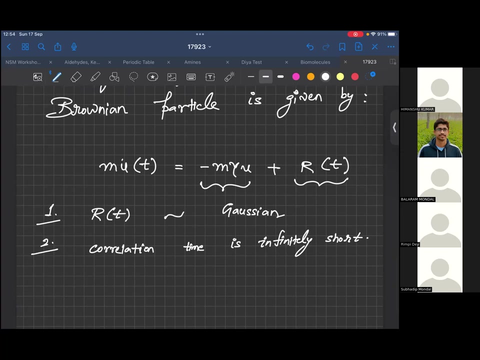 time for that, So let's go ahead and see if we can get some of the time for this question. Okay, So it's like when our particle is having a large number of coalitions, it's a relaxation time of the molecule. It's definitely going to be very, very much larger than this correlation. 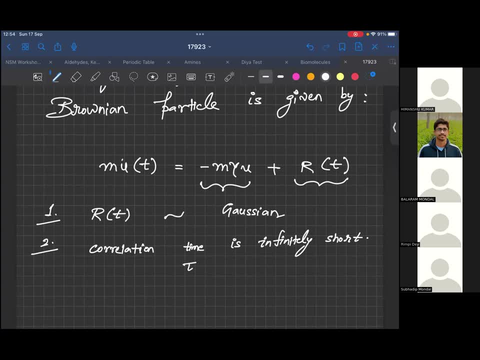 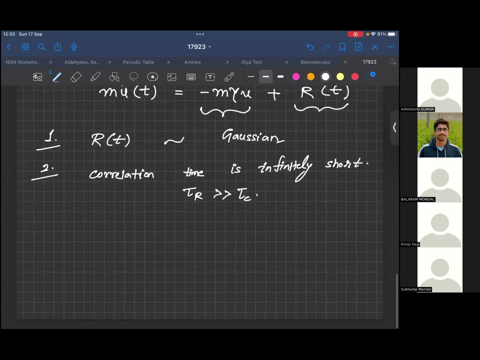 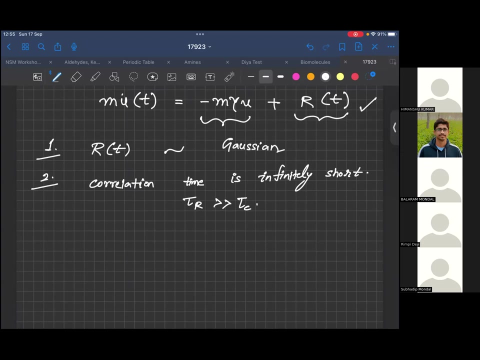 time. So basically this is the second assumption Now from this equation trip 1,. this equation constant equals Resident constant given as m square. So for sorry for my mistake, I forgot the controller. Sorry, it's gone now. 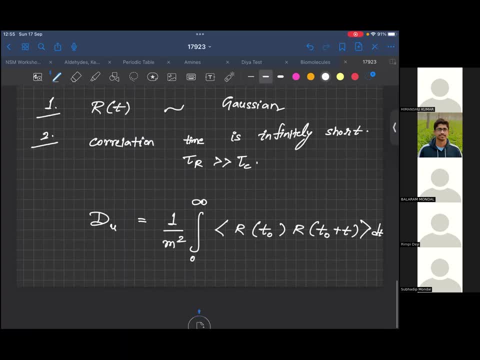 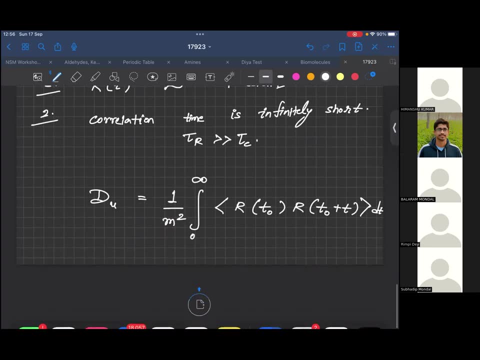 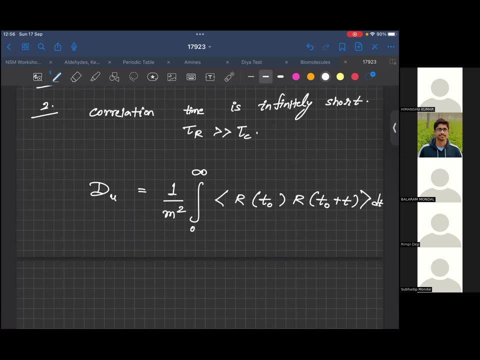 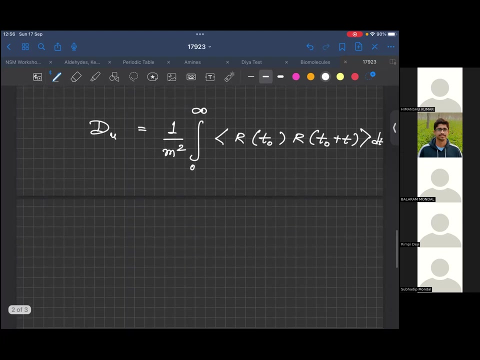 Well so? So here we can see that the random force, like the previous expression, where the mobility was given by the velocity correlation, here the coefficient- coefficient is given by the water correlation of this random force. Now, after this, just a second. Now there is another assumption. 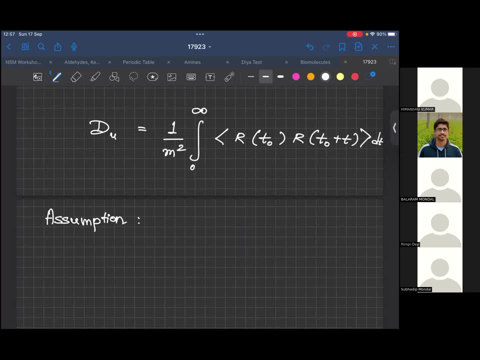 that this Brownian motion is taking place in thermal equilibrium. So this diffusion constant can now be given as gamma, by m to give it. So since it's in equilibrium, they are going to be equal to the friction constant and this thermal equilibrium, and it's here. 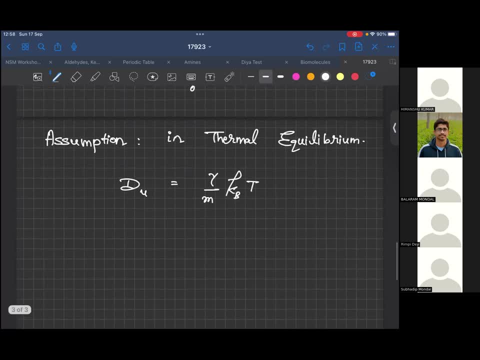 So from the previous expressions we can write m gamma equals to, and then the value of this d over. So this is the. So we can write m gamma equals to, and then the value of this d over gives us m gamma equals to. 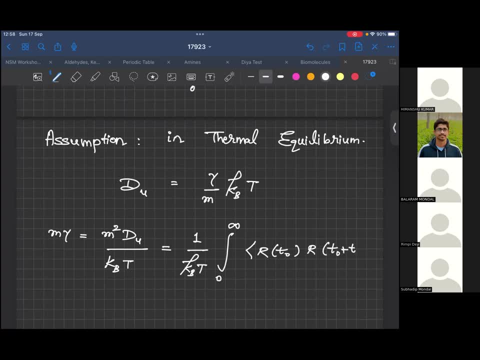 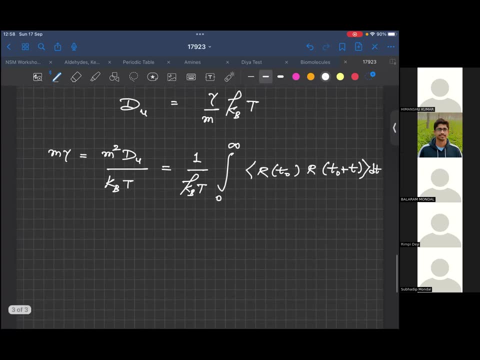 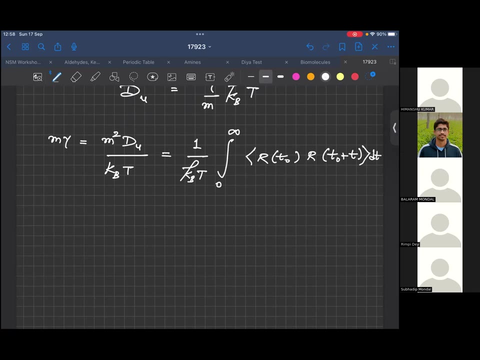 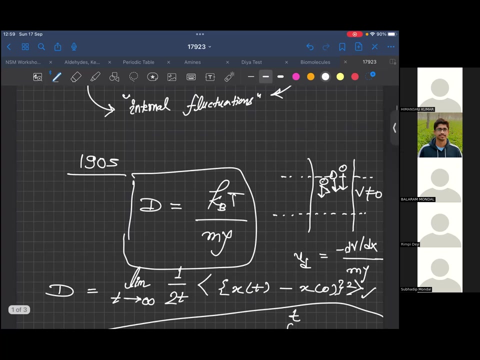 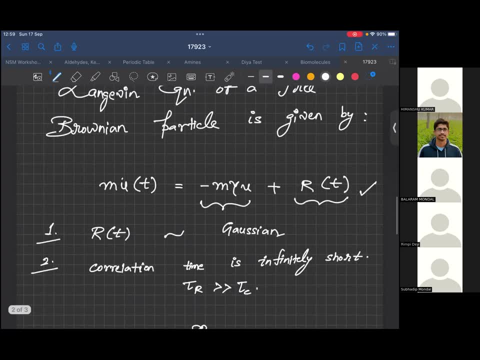 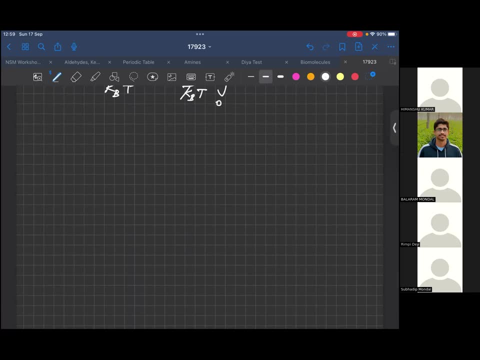 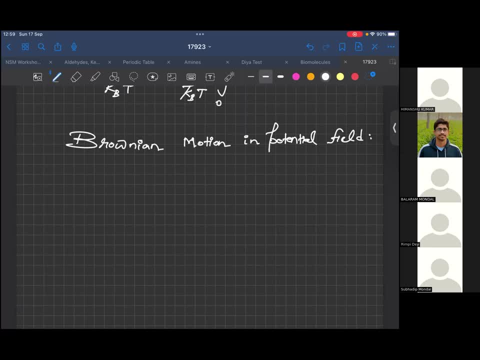 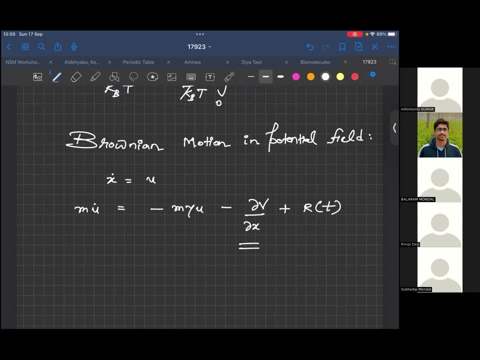 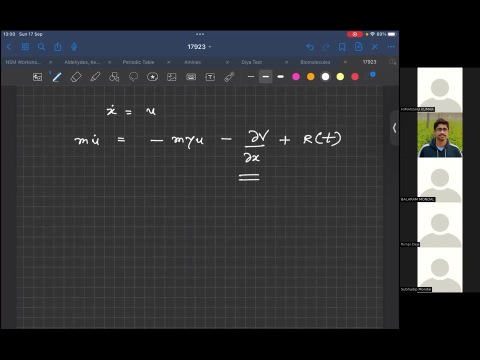 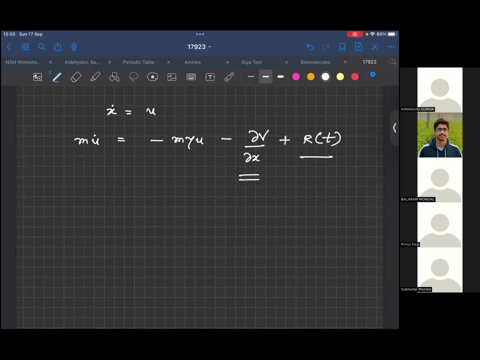 we are aware that the power spectrum or the density of states is given by this Fourier transform of this or velocity autocorrelation function. So the power spectrum for any stationary process can generally be given. as now consider why is any physical observable? it can be velocity. 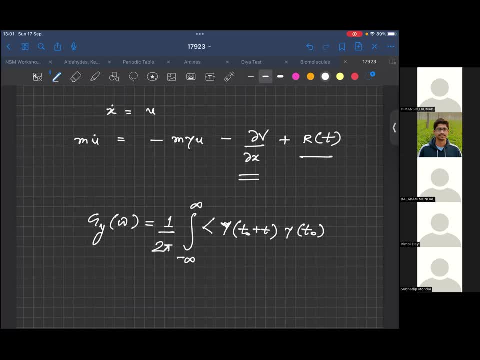 You can hear the fr�� of the state. You can hear the energy of the state. You can hear the energy of the state. You can hear it, You can feel it, You can reflect on it, You can see it, You can know your state and you can know it. 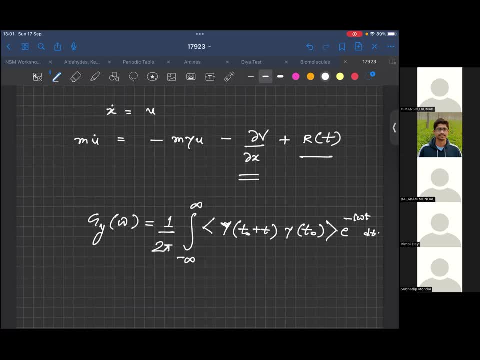 And it's also different to the way I used to see it. I wouldn't be either, And this is also very different to the balance. So it's a very different analysis, in a way we do in the past simultaneously, And we've had a lot of questions about this on a lot of different levels. 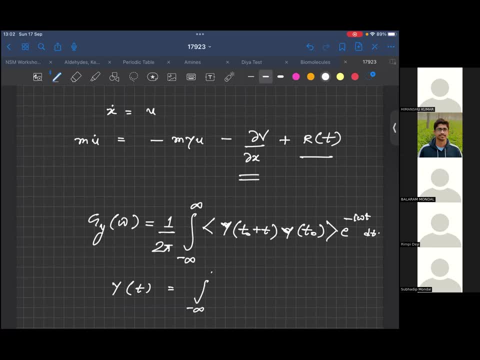 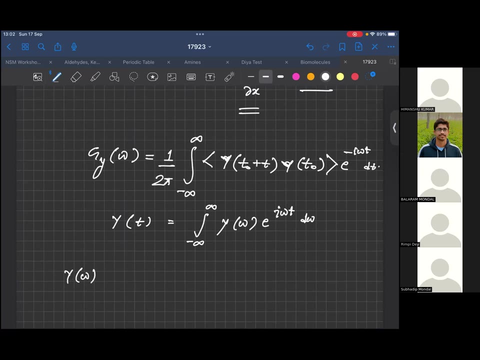 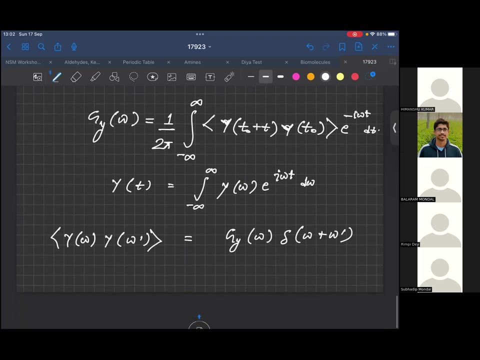 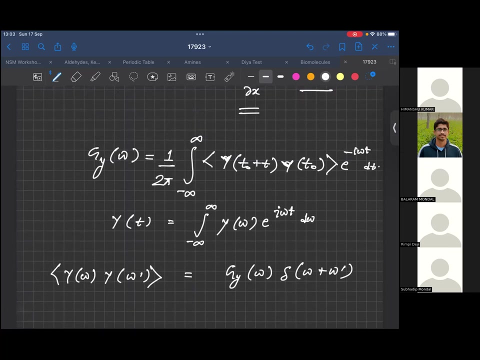 So thanks, Harris, Thank you, Thanks, Thanks, Thanks. Sticking for your transform. They have the correlation. Why do we call it power spectrum, like velocity velocity autocorrelation function? Because it tells us about the density of states, right. 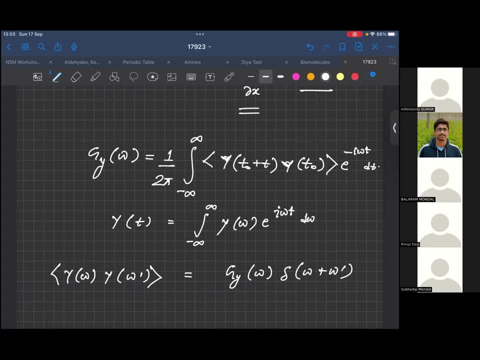 Density of states. Like you know which states are populated, Which states So from velocity. velocity autocorrelation function. how do we get the information about density of states? Origin of power spectrum, sorry, is not related to velocity, this is general term, since this: 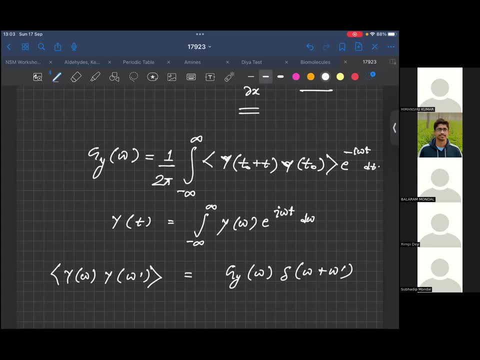 actually nomenclature is given due to the first time when this Fourier transformation is calculated. This is from the current correlation with the power response. So from there, I think this name, this nomenclature remains same, the power spectrum and we use. 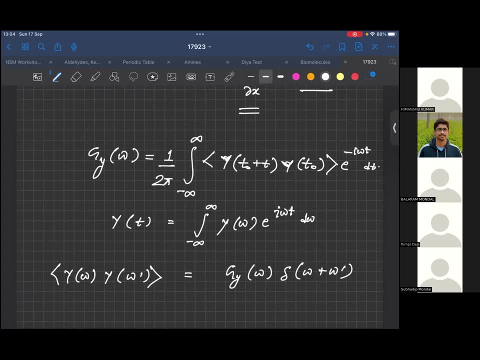 it in different, in different. yeah For any linear response like structure in the like in the current setup, like LR right, Yeah, Yeah. So I mean the thing is that, for example, in the current setup, so in the current setup. 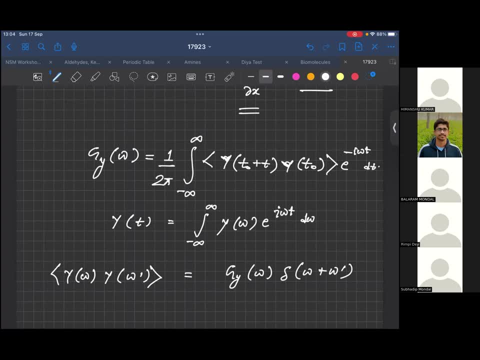 we put in a power number. which scheme That was we forget? yeah, in the current setup. So they actually computed the power power response function. So from there they get this type of expression. Yeah, I, I actually the connection. 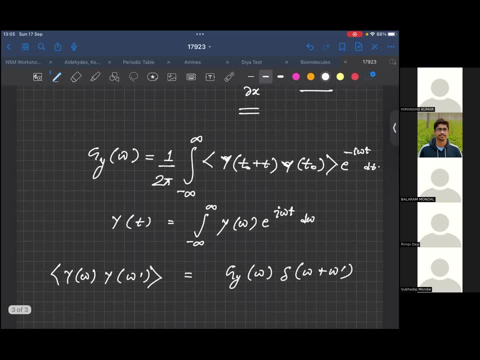 Yeah, And my second doubt is: how is it different from the dipole, dipole autocorrelation function? Which one? The penguins? The penguins, right, like that's a different physical, observable, right? yeah, like what is different, like velocity. 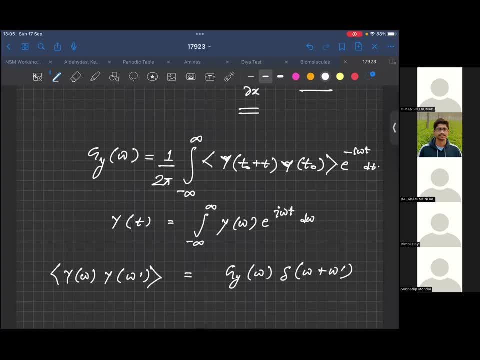 autoconversion function. Fourier transform, we just call it power spectrum and we also say to get the accurate dynamical information from spectroscopy, we should compute, dipole, dipole. so why? this is like, what type of information is missing from the velocity, velocity, autoconversion? maybe this is general. now, why you make, why you are. 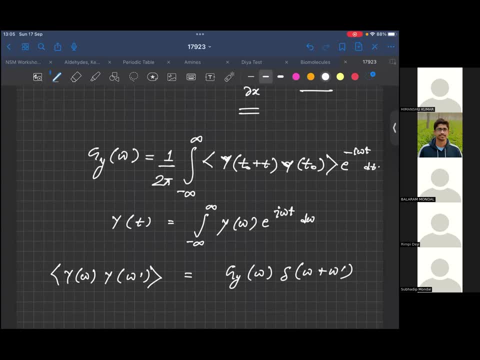 for general observability. why? yt means any physical also, like it can be moved here. velocity and dipole, autocorrelation are exactly means if we, if we write the dipole in terms of coordinate and charge, write it down. so basically, if our dipole, if we approximate, 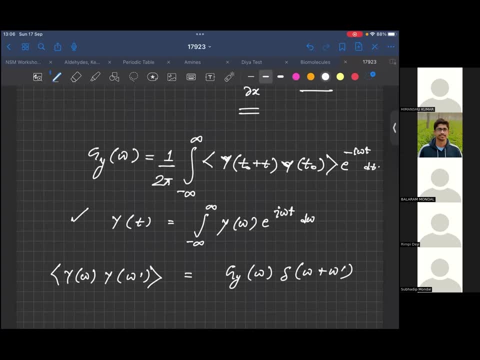 our dipole function and we write the dipole in terms of coordinate and charge as a linear function, then will it be accurate or not? yeah, if we means yeah, so that that's the real, real dipole. no, sorry, linear dipole function. so if you write in: 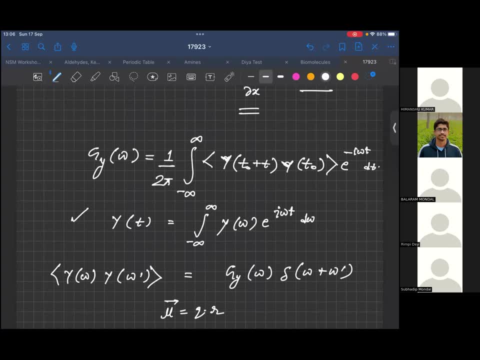 this form, then i think the velocity, velocity, autocorrelation and dipole, dipole, autocorrelation will be exact, right, yes, yes, it will be exactly means connected with that. uh, charge to yeah, to the charge, yeah, yeah, but does that answer your question? yeah, yeah. so basically, i wanted to know that, uh, how these two functions are connected, or? 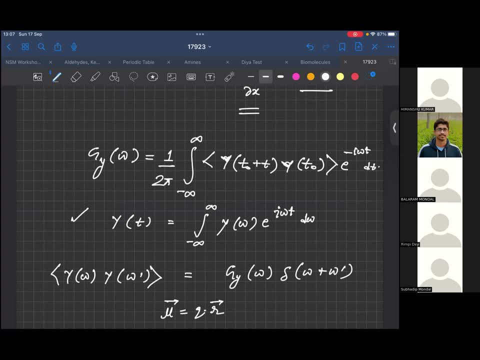 not, or how different it is actually. but i thought you were asking, like: why do we get the exact response from dipole moment and the power spectrum from the velocity function? No, no, We also compute power spectrum and dipole-dipole autocollusion function, right? 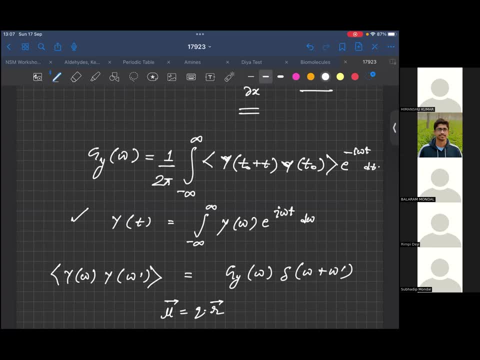 But what type of information are we actually we are missing from the power spectrum and what type of information we actually get from the dipole-dipole autocollusion function? That's what I mean, That's my concern actually. So, basically, if our dipole function is linear, 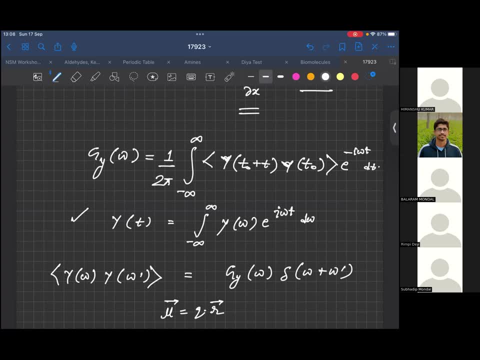 if we approximate our dipole function as a linear function, then we get similar type of information from both power spectrum and dipole-dipole autocollusion function. But if our dipole function is non-linear in nature, I think then the spectra will be different. 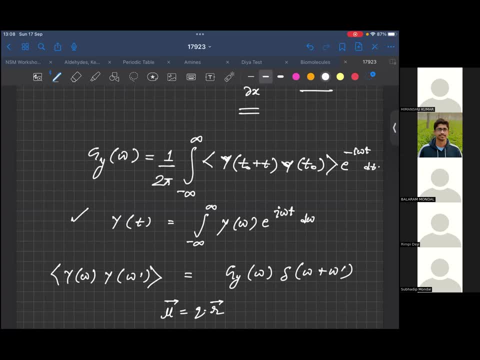 or information will be different. I mean see if we cannot simply write down it as Q into like: even if you have water, we approximate it by linear function. but it means in general there is no simple charge multiplied by position of oxygen, like that. 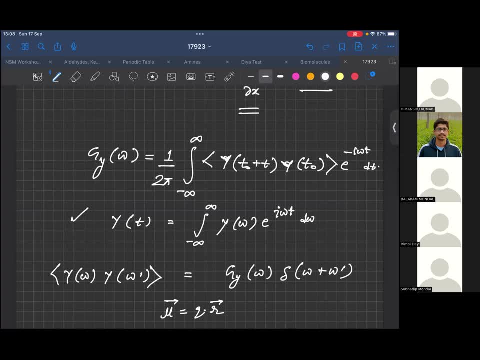 So they are this expression, they are these similarities does not be easily visualized that dipole-dipole and velocity-velocity, but for force field, where for point charge, there you can means exactly see that dipole-dipole and velocity-velocity are similar with the charge factor. 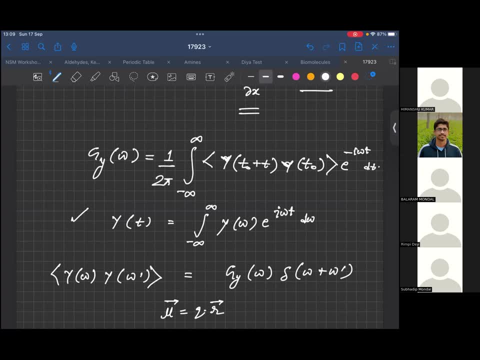 And the information means velocity-velocity, we can get to know the every motions in the system, but for dipole-dipole, we can get to know that which motions will be interacting with the electric field, with the AC field, oscillating electric field. 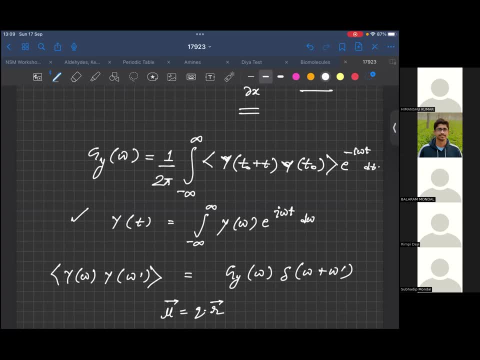 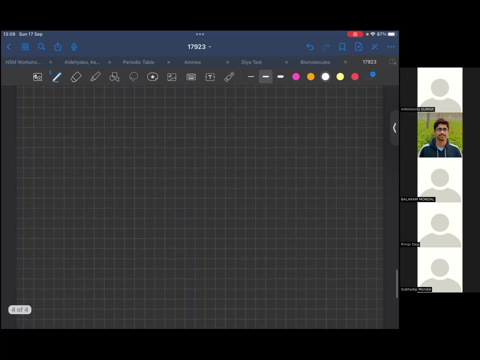 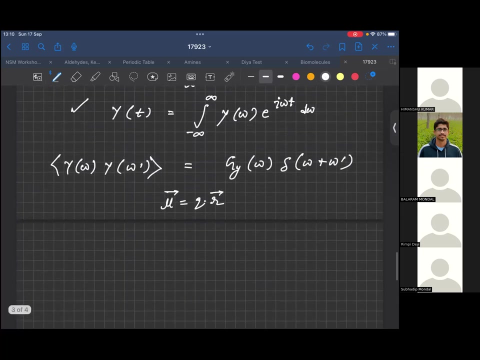 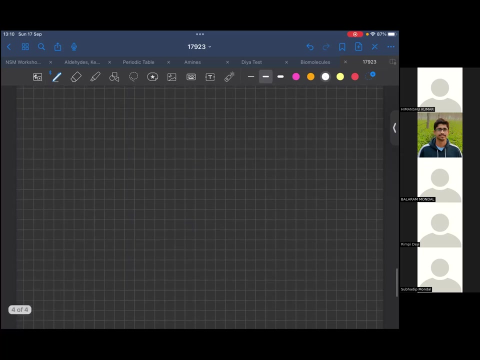 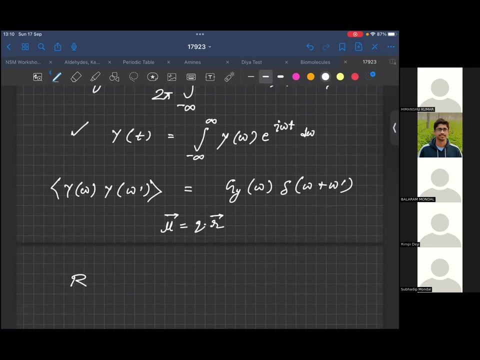 So two informations are important means for that sense. One give the full vibrational information and one gives the active vibrational information. Yes, yeah, okay, So let's just go ahead. We got that very short, so let's just put. 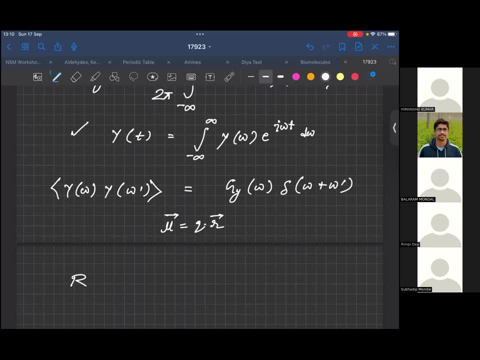 And just one point- Actually I was talking to someone like she was like she's doing surface spectroscopy, like H2 dissociation on some surface- silica surface or the palladium surface- So they actually compute the velocity-velocity autocorrelation instead of dipole-dipole autocorrelation. 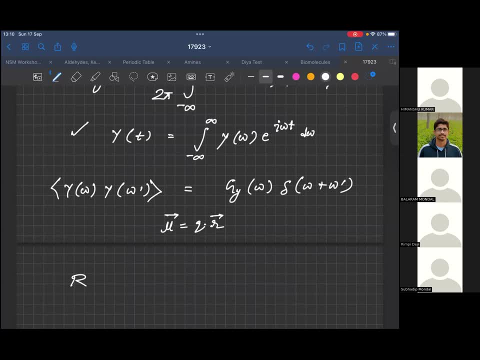 I asked her why they are doing this. She answered that if our dipole function is Q times R, so that's why I didn't quite understand that. but yeah, I don't know why they are computing velocity-velocity instead of dipole-dipole. 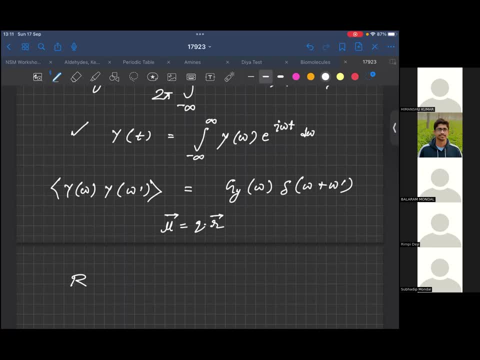 I think they tried to say that it is similar means dipole-dipole velocity-velocity with that approximation. But when this approximation does not hold too much, like if we have metal, then this kind of thing would be disaster. It's more delocalized nature of the electron. 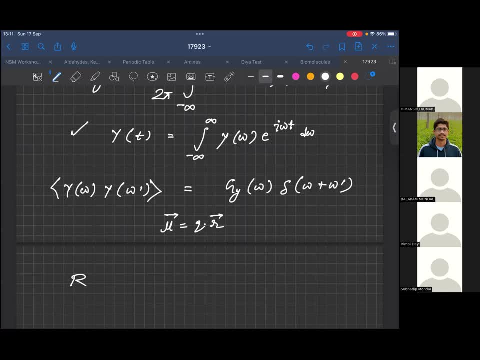 We could less approximate? Yeah, but he said it's on the surface of metal only, right? Yes, on the surface of metal. That's why I think, yeah, I think that it is not easy to get dipole information from metallic surface. 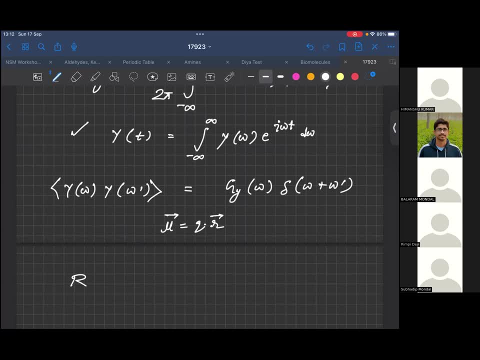 It is still under. Okay, She is here like in IDK. No, no, Okay, She is in Peter Salfrong's group in Berlin. So, okay, So you do actually this kind of surface spectroscopy, IR spectroscopy for the molecule dissociating on the surface. 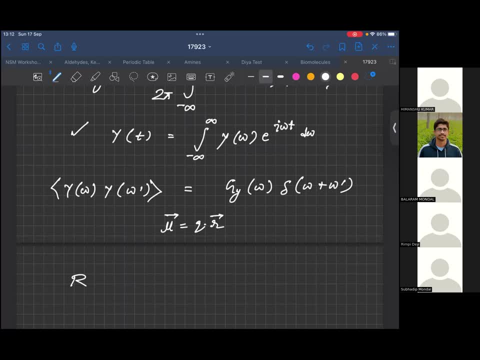 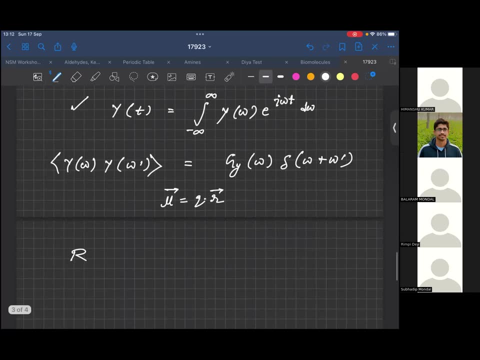 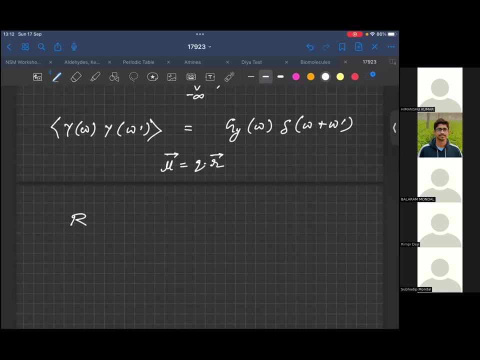 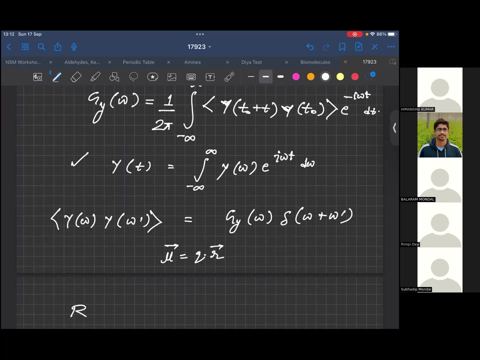 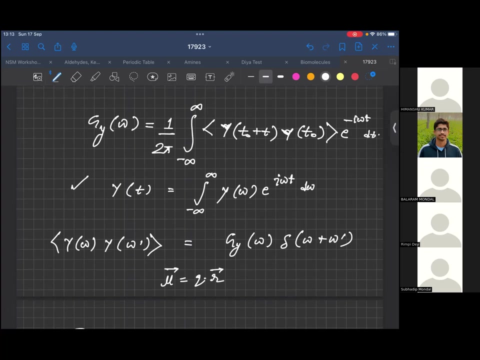 like this for reactive system IR spectroscopy. You can just look into that group And RIMP where if you put back- that means if you put that uh expression of Yt into the expression back- then you get the double Fourier. transformation means G omega. 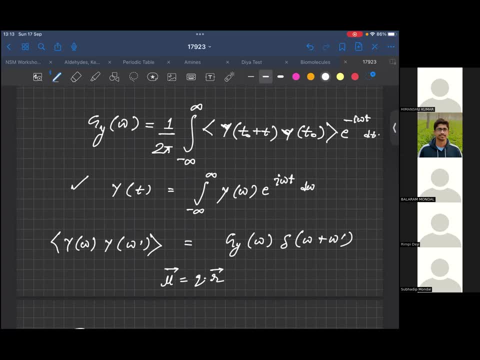 Yeah, And we calculated from Y, omega itself using this double Fourier. Yeah, That is one theorem means one can efficiently calculate because Fourier transformation one can efficiently calculate using first Fourier transformation. Okay, It is early and also very accurately. So this many people do this kind of trick to calculate this power spectrum. 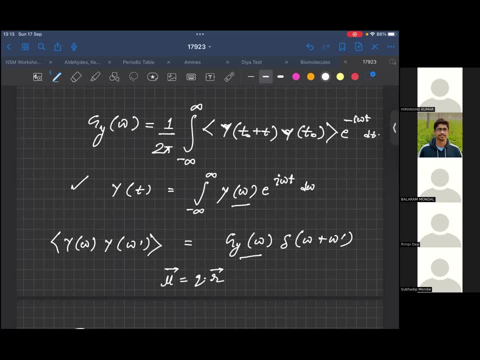 What's the significance of doing this double Fourier transformation? No, there is no means. it is same mathematically, but numerically or in terms of That's possible, In terms of calculation, if we calculate means, if we can, because it is finite. 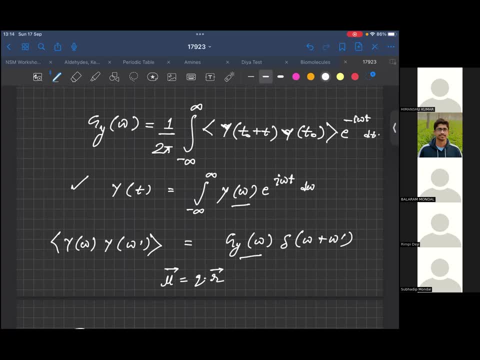 this all the correlation function will be finite. So whenever we truncate it, error comes from this truncation part. Okay. But instead of this, if we do this, Fourier transformation, okay. So Fourier transformation actually um most efficiently, uh. 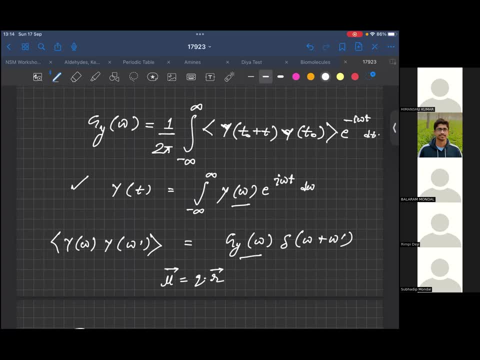 approximate the truncated part also Okay, Okay. So that's why many people prefers this way. means double Fourier transformation to get this power. So there is a theorem, no cringe and theorem in spectroscopy. spectroscopy people use. what theorem cringe and uses? see the barbary. 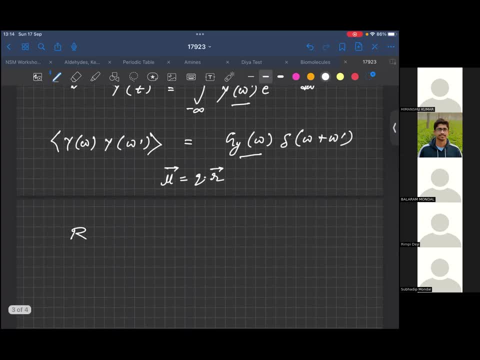 Okay, Barbara cringe and paper, paper, Okay. Okay, I'll look into that. There is a square of this function and then put it on. Okay, So uh, in this expression, if I just replace the physical quantity by by our random force, 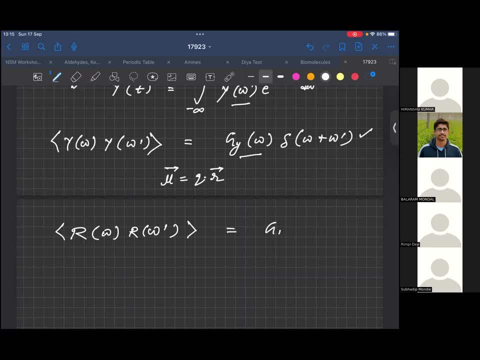 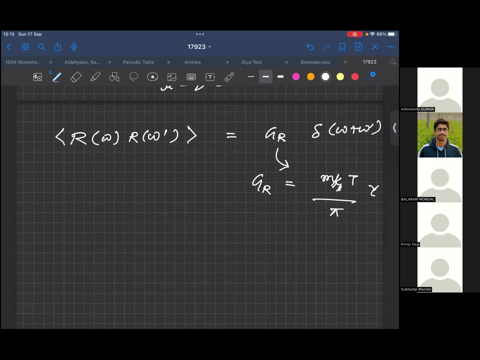 then we're going to be given us some GR and this GR is given us right. so from here we can say that the power spectrum is actually determined by our friction. Okay, So we're going to be looking at the dz to answer it so we can take the resources from the heat and the energy to. the heat is determined by the temperature of the system. that means the resistance to the system actually tells us how the states are going to be populated. 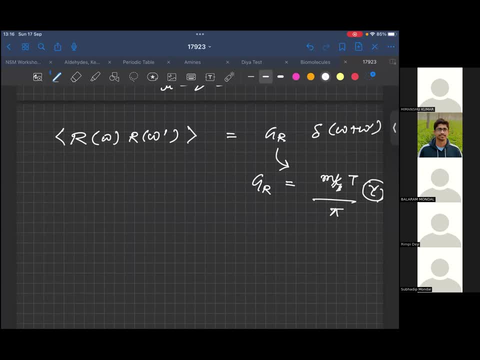 And how is the energy going to be dissipated? the thalminology, the microscopic thermal energy. So this thermal force, which is the r, is actually the result of thermal fluctuation. So this was actually given by McQuist theorem in the year 1928, where he showed that random. 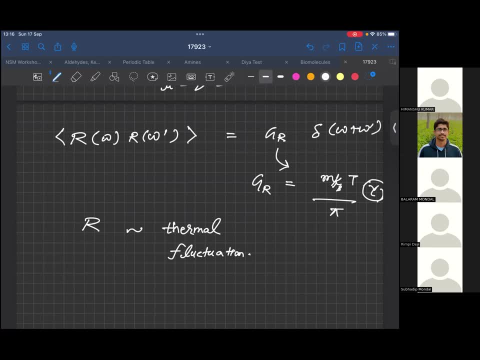 electromotive force, EMF, appearing across register is determined by the impedance, and impedance was actually connected to this external electric field that we have applied. Actually, the paper that I have chosen for today's talk is too long, so I will be just writing the equation here, because won't be able to derive so much right now. 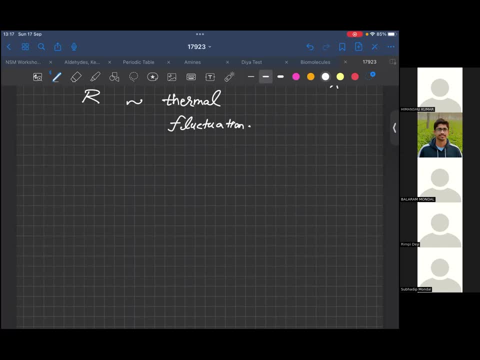 So in equilibrium this velocity autocorrelation is the mass square e to the power minus kappa into t. Now if we differentiate this, we can see that the velocity autocorrelation is the mass square e to the power minus kappa into t. So 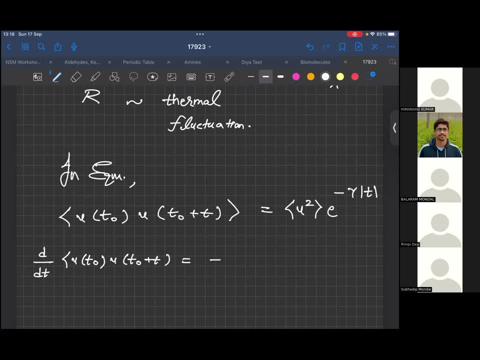 let me write this u square as t zero plus t, So let me be going to be minus comma and then then write this u square as t zero plus t, Like just using this expression here, or definitely take it in zero. Now I'm going to write this expression here, or definitely take it in zero. 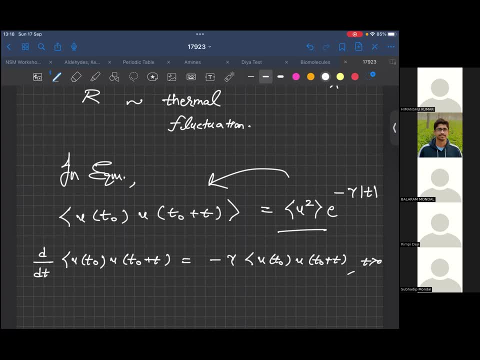 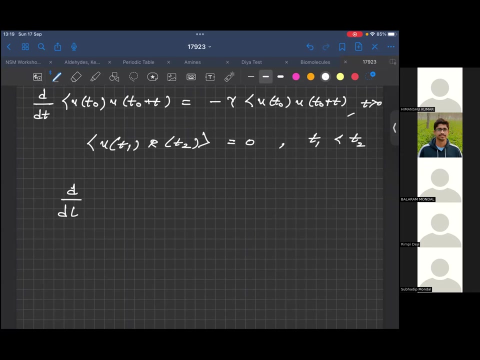 Now we will take this expression here. Now I'm going to take this expression here. So the correlation between this velocity and any random function should be zero. provider: here t1 is less than t2, so this means that d of d, t0, initial time- we differentiate with. 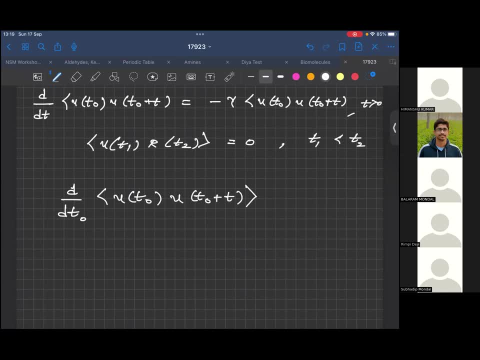 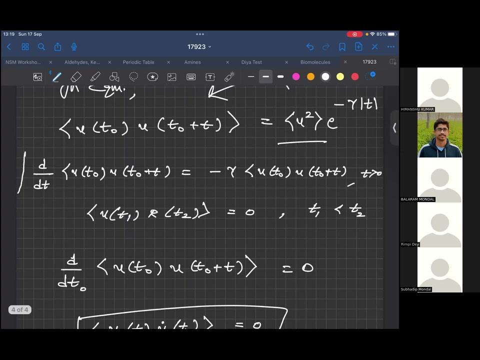 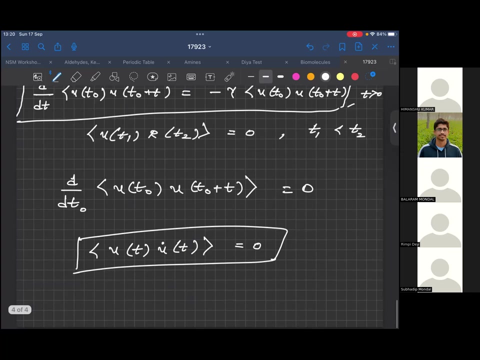 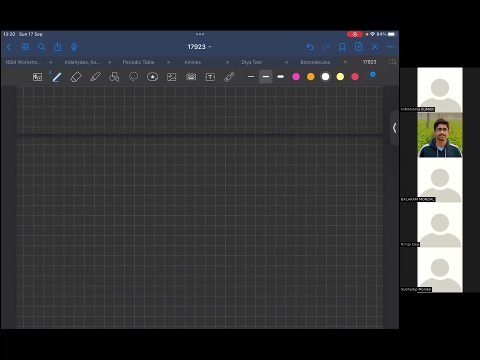 respect to initial time should always. this correlation should be zero. so we say it's going to be a stationary process. however, we say this equation is actually contradicting the above equation here. so in the year 1965 and moody, sorry, moody in the year 1965 and kubo in the year 1966 individually. 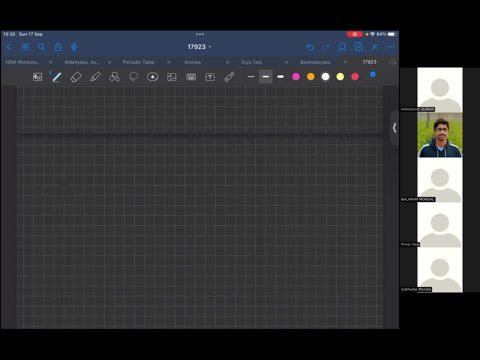 uh, gave a natural extension of this nanzibian equation where they said this: so, so just get this most deep. okay, let me change this to the up. So this part is our frictional force, this is our random force and this is our external. 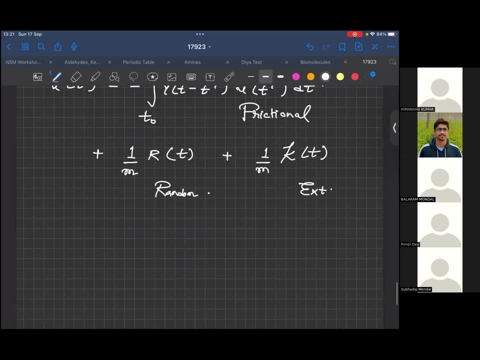 force. So this gamma t, actually the frictional force. it represents the retarded effect of the frictional force And we assume that the average random force is going to be zero. So in short time velocity and this random force correlation is going to be zero. but obviously 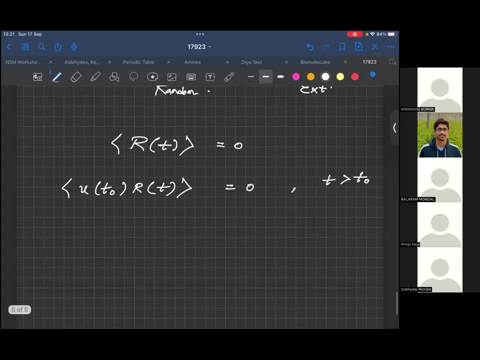 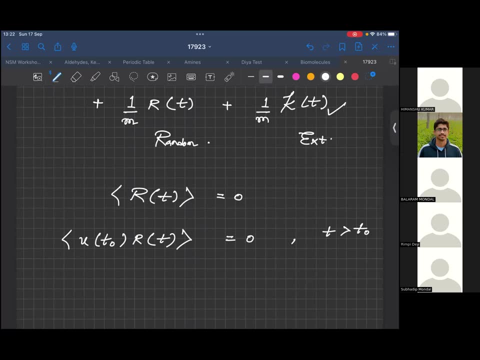 t greater than t zero And it does not depend upon our external force kt. Now, if we consider that this k is a periodic external force, so it will depend on k zero course of an omega t, Then this equation this modot: t: 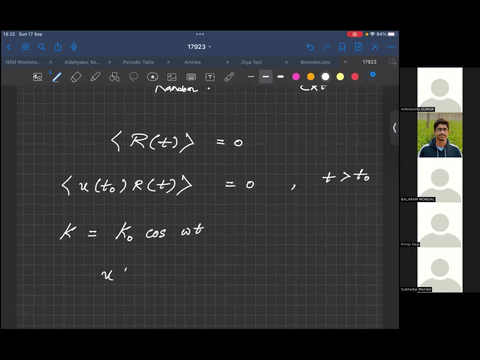 And it is given as k zero e to the power i omega t, Where mu is our mobility? And it is given as k zero e to the power i omega t. And this is our modot, And this is our modot. 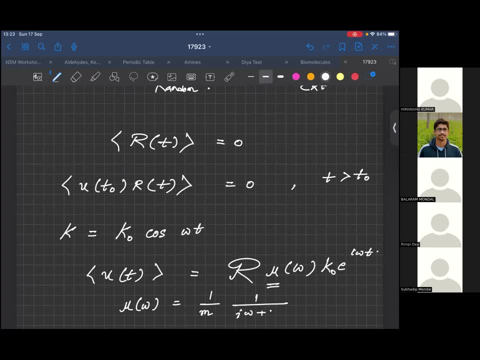 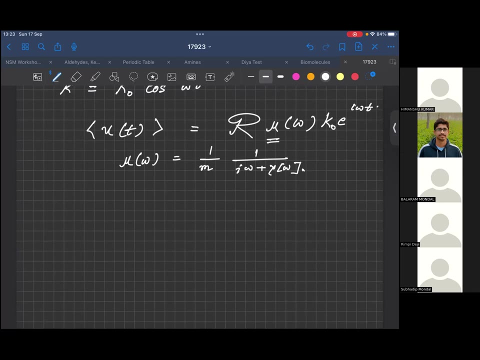 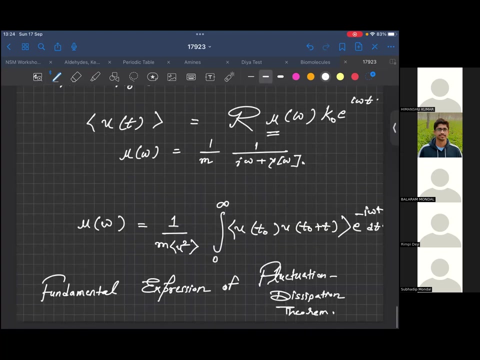 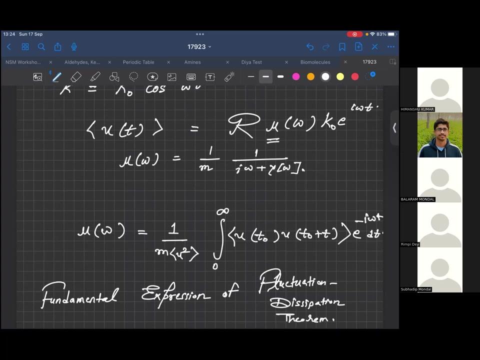 And this is our modot Thank you. So this is the fundamental expression of our fluctuation dissipation theorem. So this is the fundamental expression of our fluctuation dissipation theorem. So this is the fundamental expression of our fluctuation dissipation theorem. 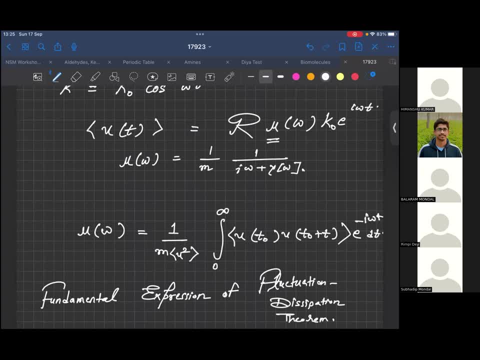 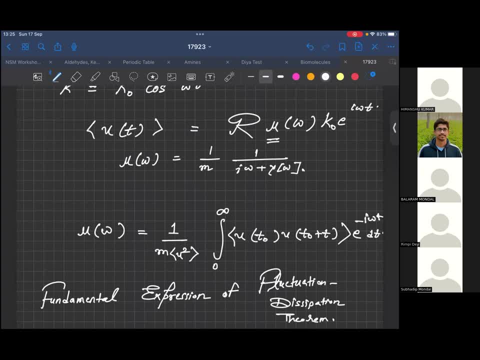 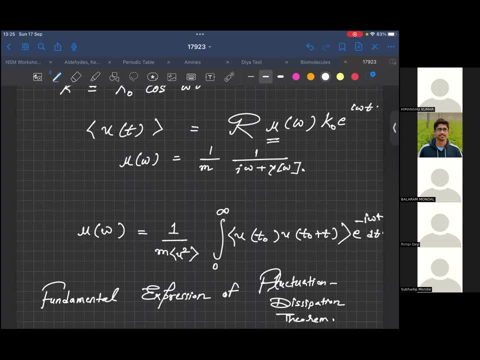 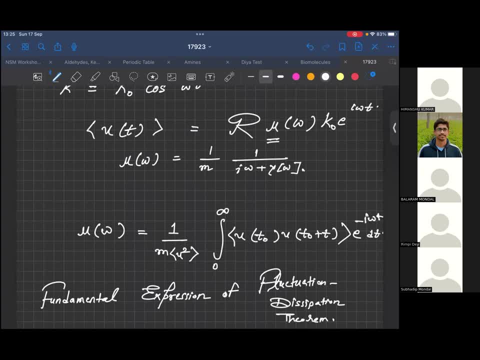 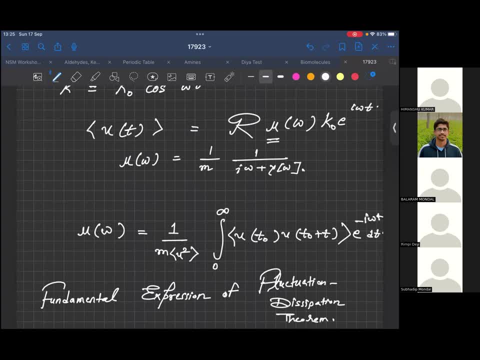 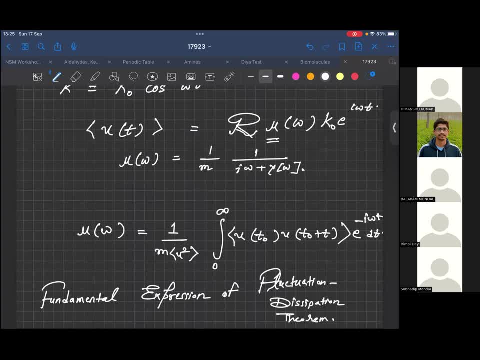 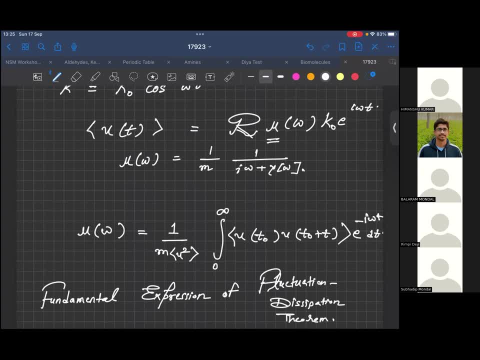 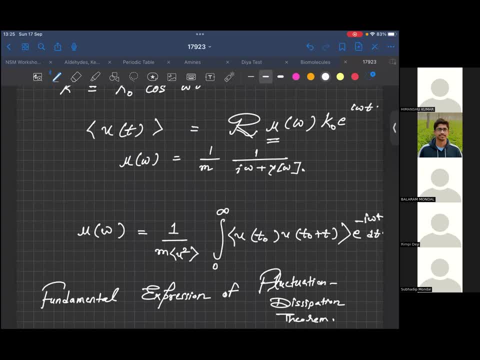 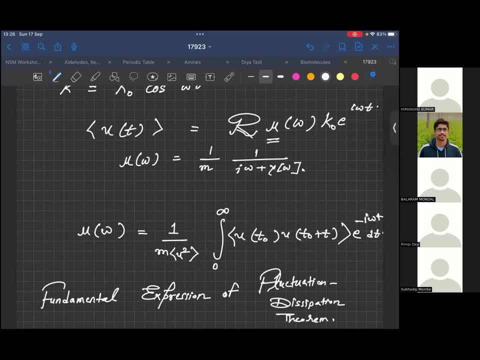 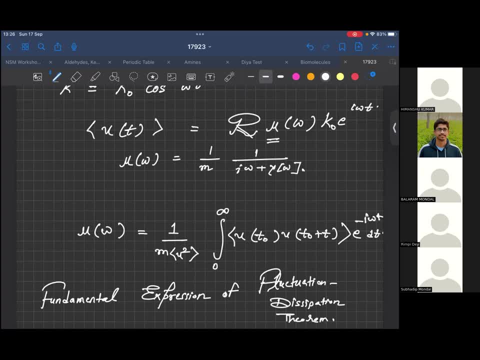 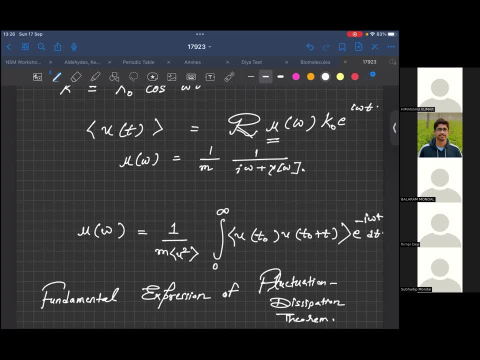 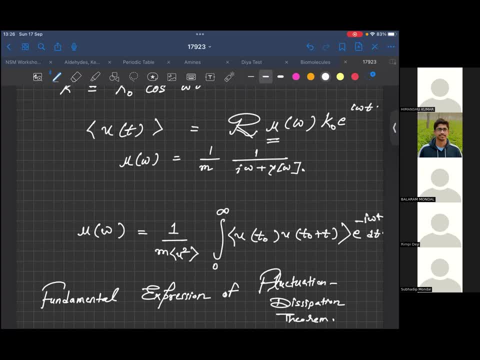 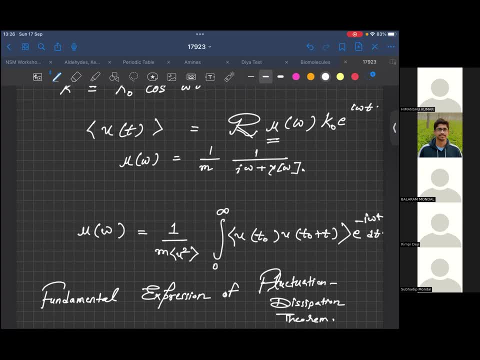 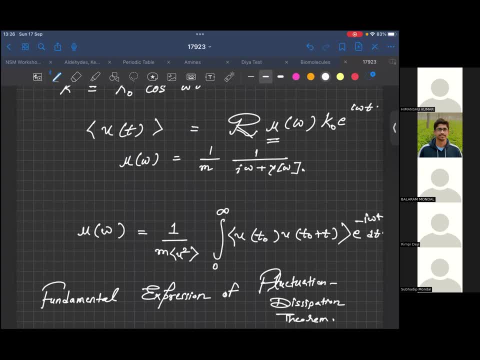 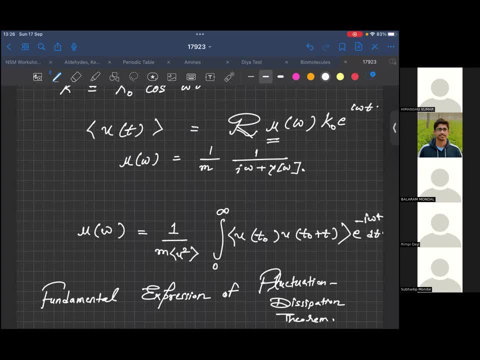 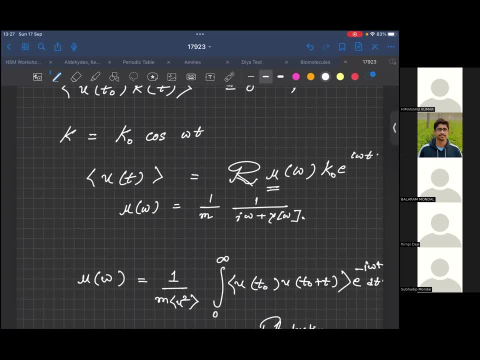 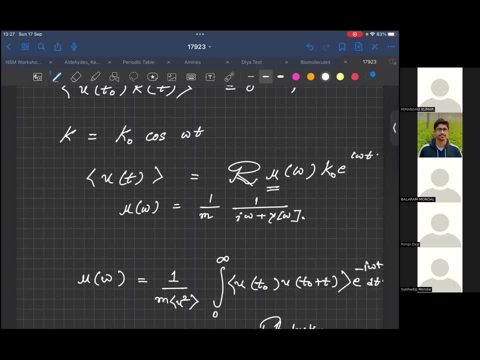 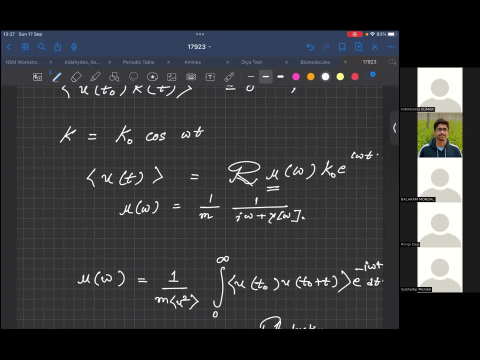 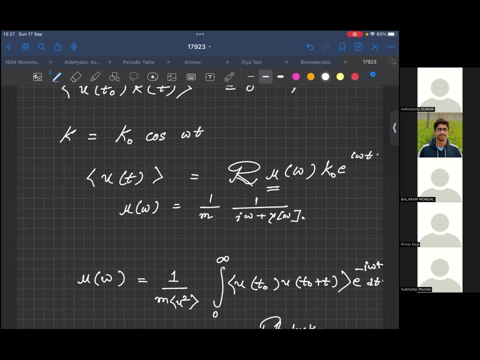 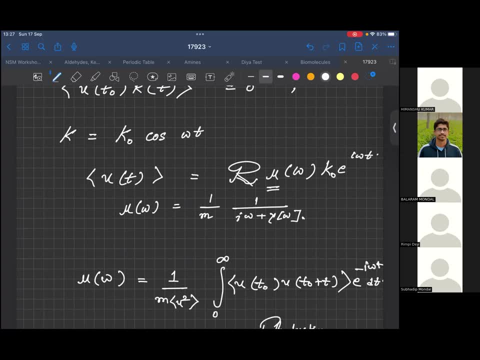 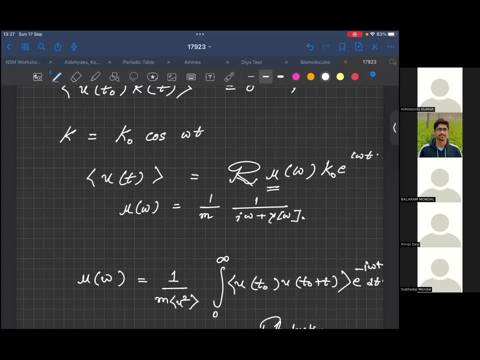 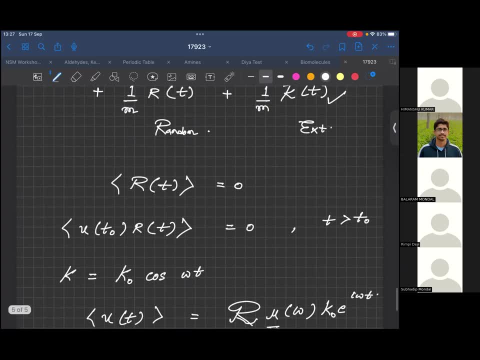 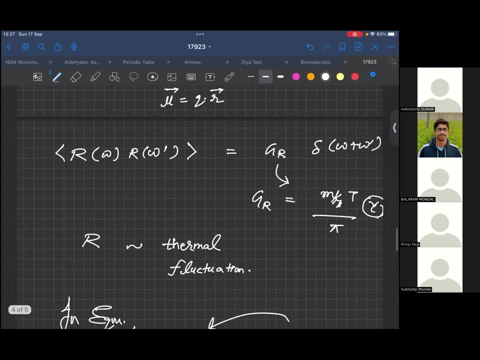 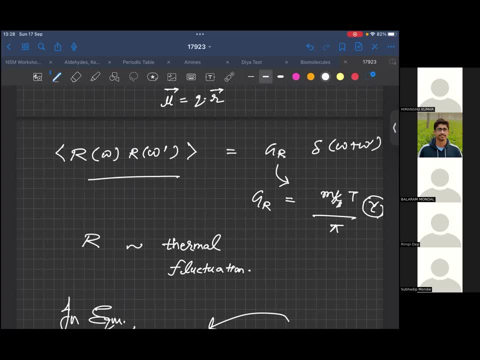 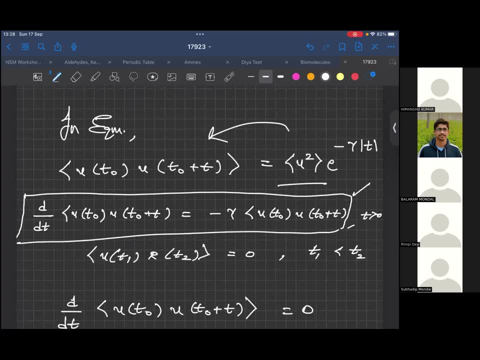 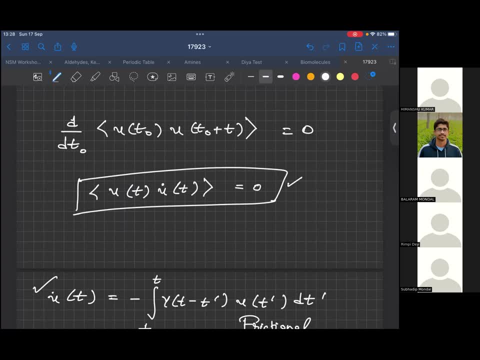 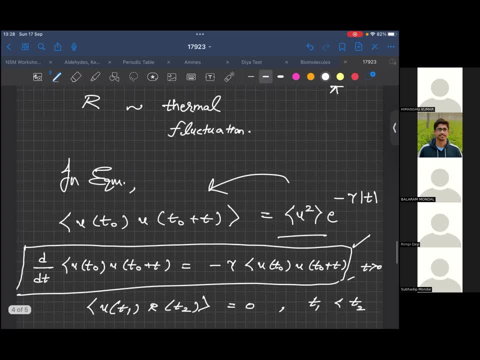 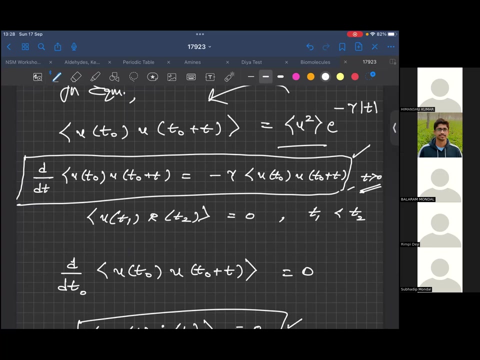 where did it go? yeah, it cannot be zero for any time greater than t, greater than zero. so sorry, what was the question again like? where did the random force correlation go? r, t, r, t 0, r, t 0 plus t means it is delta function in the emplaced assumption, but in 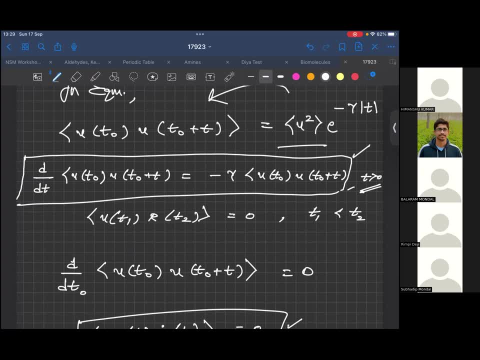 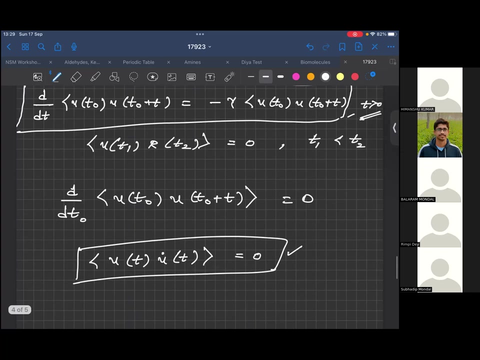 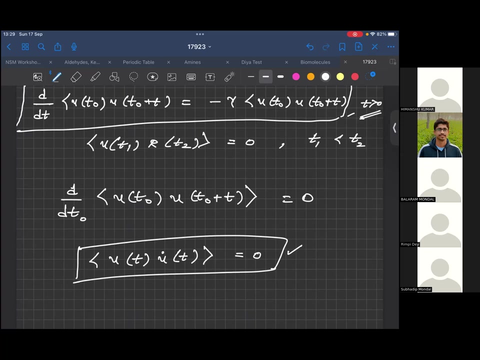 that specific case, what would be the expression? i don't know what to say, i don't know actually, sorry, i don't know, actually sorry, i don't know actually, like for your stationary delta correlated noise and for Markovian process. so the fluctuation distribution theory you get. what is the expression like? 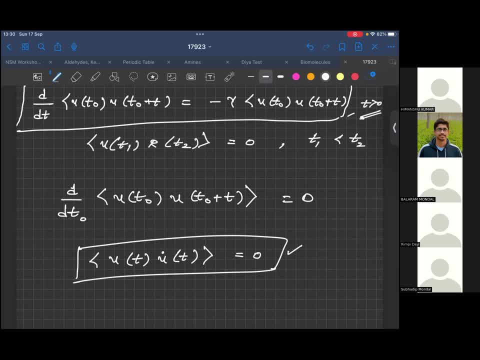 that is r of, if you any take your physical observable as r, and it's going to be r t 0. r t 0 plus t and then 2 pi g of r delta of delta, function of that t 1 minus 2. yeah, yeah. so basically it will be like r t 0 plus t and then 2 pi g of r delta of delta. 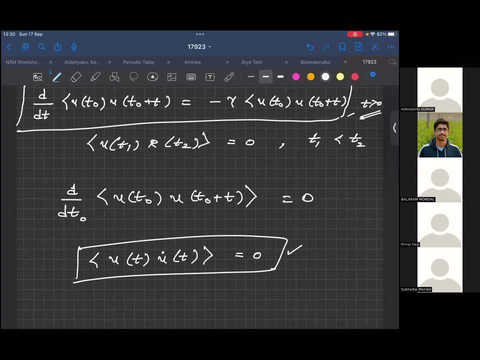 and like k b t equal to m, gamma something, something mm-hmm. so that's that is for markovian, stationary markovian process, stationary and delta correlated noise, mm-hmm. that is for um. but station Sebabad is this one? yeah, and that in that was also for stationary process. 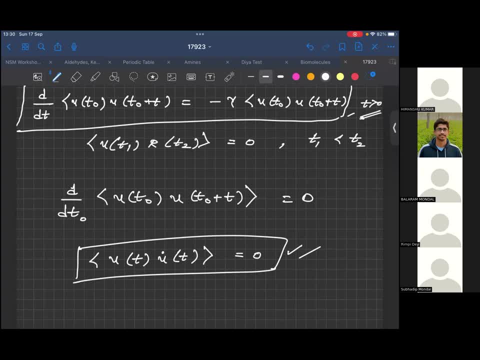 yep, okay, that one is for results here. very much, okay, Mundi- This is the motivation value. Delta correlated noise: Delta correlated noise- okay, yeah, and now here, what's the difference like? is it Markovian or is it Markovian? it is Markovian also right, because Gamma is constant. 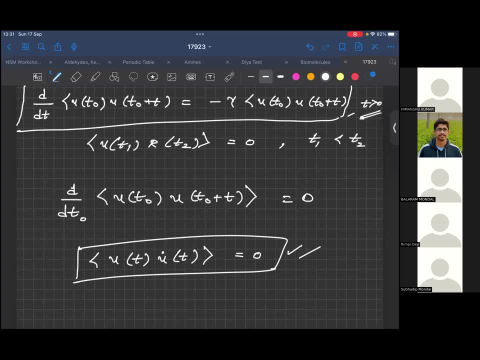 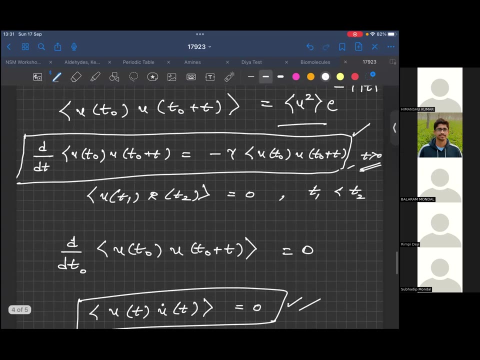 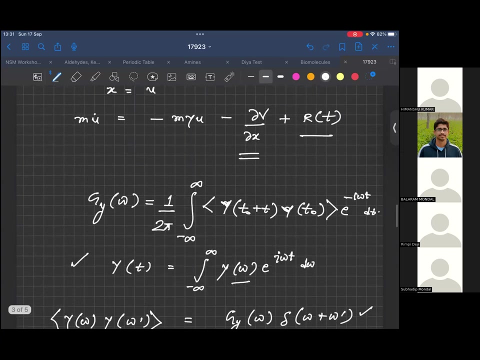 here, or Gamma is, Gamma is constant. yeah, so that means this is Markovian and your noise correlation is also Delta correlated here or not? so the in the previous one, like where I gave this R of Omega and R, where there was one assumption that we took, now that is the Tau of 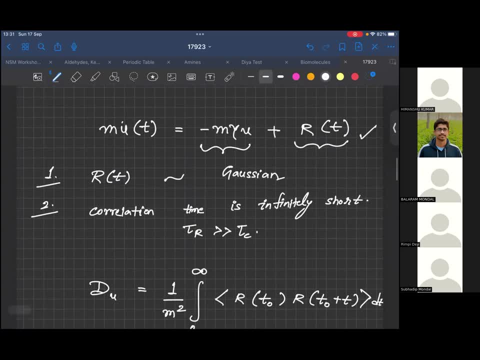 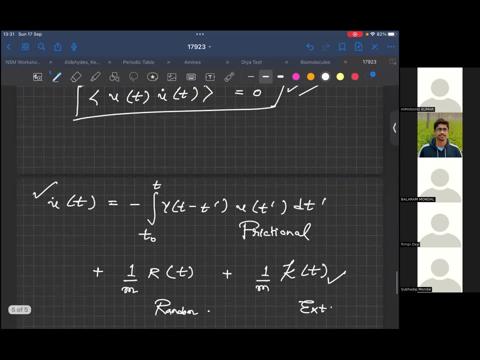 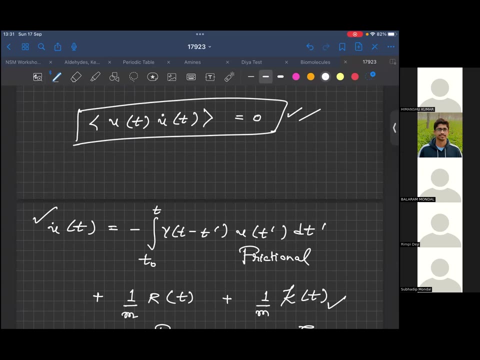 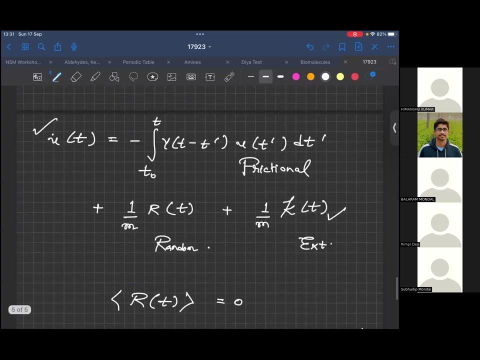 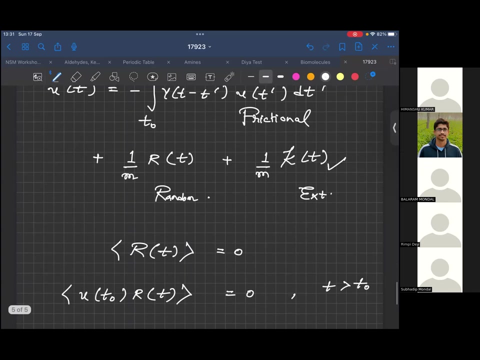 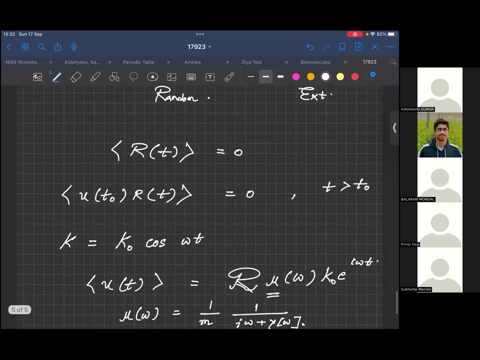 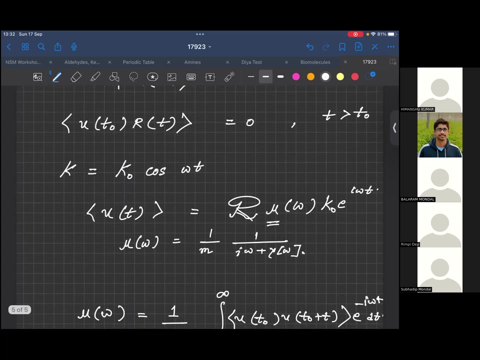 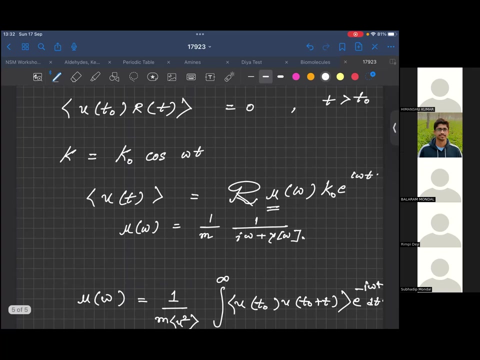 R is going to be greater than this. this assumption was there, so this assumption is not valid in the case here. that's the difference here. but how is it making sense? okay, just scroll down, scroll down. yeah, scroll down. so okay. so so basically, Mu Omega is the mobility right: mobility. 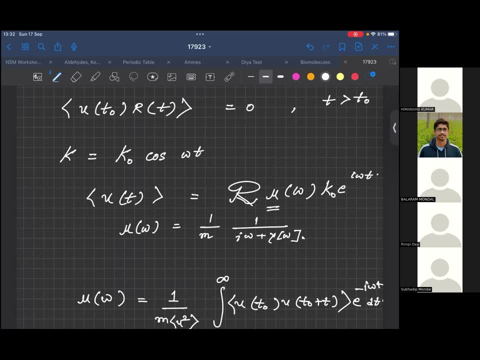 so mobility is relative to the velocity. velocity correlation: chordian transform: U is velocity, U is velocity. you know, that's the, that's the doubt in the previous expression, like in the mu omega expression. so omega you have written mu, omega equal to one upon m times one divided by i, omega plus gamma. 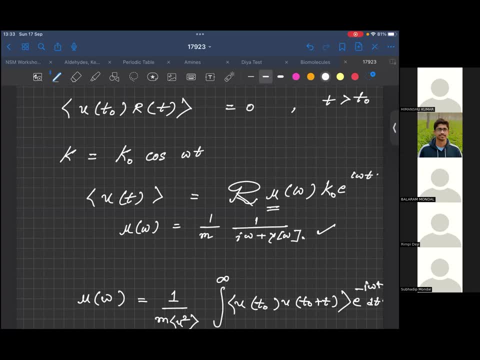 has a function of omega right, but this is true only when. when gamma is non-markovian, like gamma is some time dependent right, history dependent gamma. if gamma is our constant, like for markovian, then it is just a constant right. but, uh like, from the paper from where i have been discussing this, they have written that 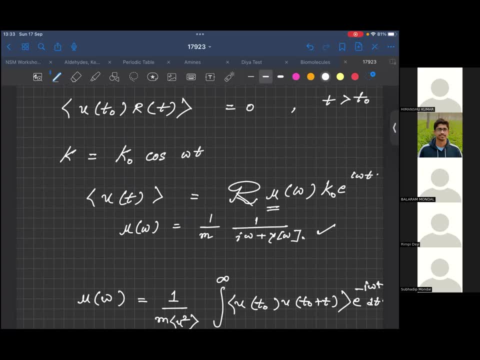 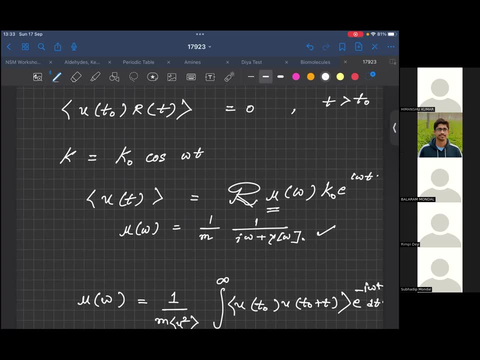 uh, like for the, where i said that this assumption is no longer valid here. so they have written uh for the generalization of brownian motion theory to random motion of the particle which is not necessarily heavier than the particles interacting with it. so this means that the time scale of the molecular motion is no longer very much shorter than the. 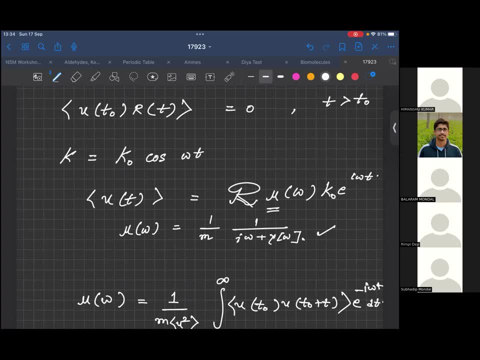 motion of the particle under observation, so that tower that is not gets valid. yeah so, yeah. so, in order to meet this requirement, we have at the same time to abandon the assumption of constant friction, all right- and to introduce generally a frequency dependent friction. yeah, that's right. so that's, that's basically. it is a non-markovian process, uh, general it. 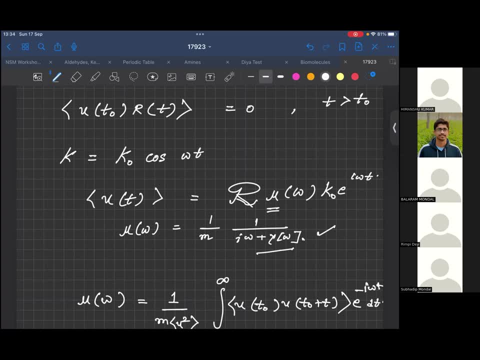 is from derived from generalized lentiment equation, right? yeah, that's that's why i have a. it is normal and it is also written in the expression of land of any question. yeah, it is from generalized engine equation. where did this random correlation go? random correlation, i think there is no specific there. 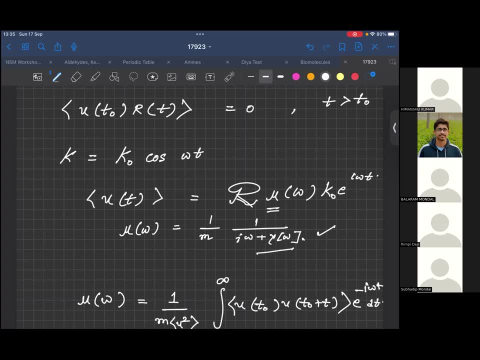 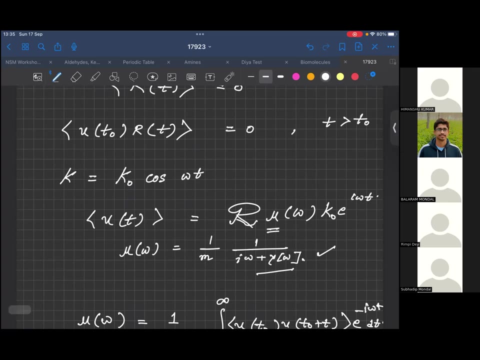 is. this is the only assumption you made here- means, uh, our average for random part? yes, it should be zero. yeah, this average random is zero. okay, yeah, and this correlation with random, uh, velocity is a later time. yeah, this is zero. this is, yeah. these two are the only. this two are. these two are the assumptions. 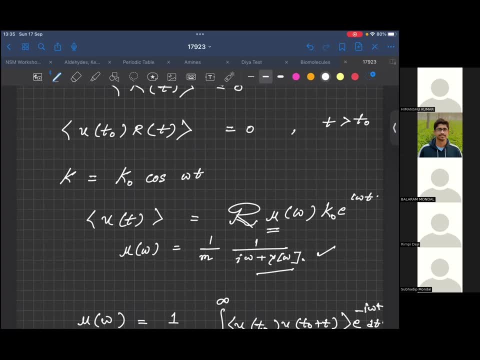 only assumptions. okay, and the great gaussian property assumption remains: okay, random will be gaussian, but not neither. not delta function. no, it's not mentioned. yes means i am thinking if delta function, whether this delta function and these markovian things are connected or not, is because you already made. 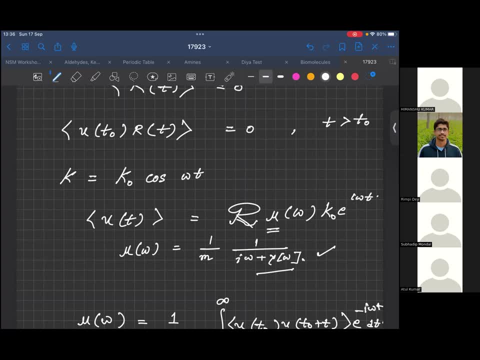 the friction non-markovian means history dependent. so friction to be history dependent. the random noise means can't be zero delta function because uh, friction and the random part is connected by fluctuation dissipation theorem. okay, So one is extreme and other is not. that is not possible. So I think this is the reason. 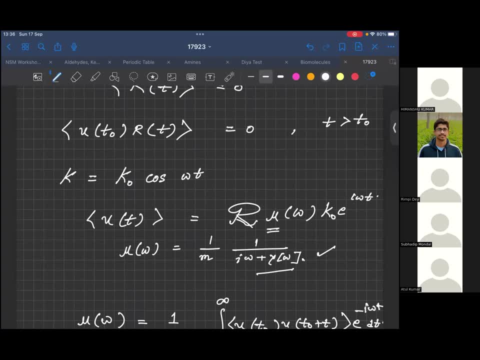 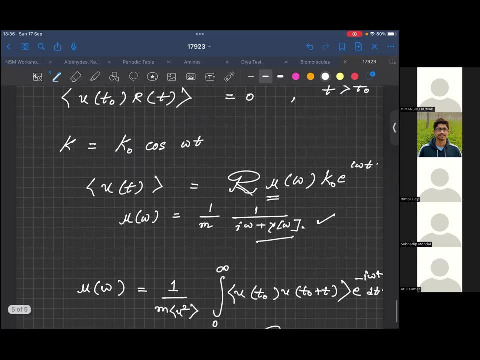 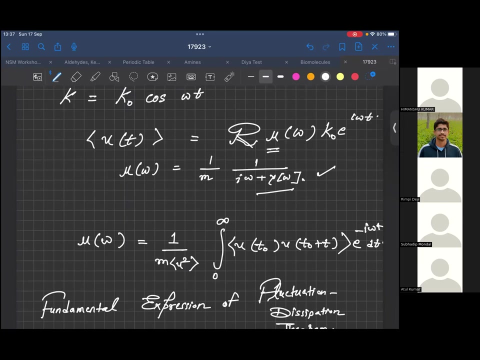 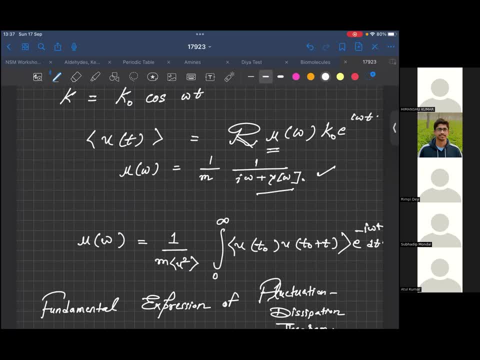 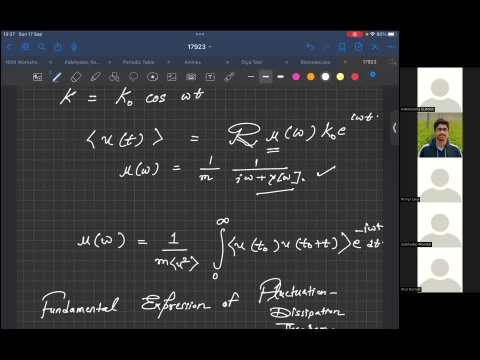 friction, This bordering this line with the history, dependent friction. So yeah, these will explain the means. bordering part means, otherwise it is earlier, it will be delta spike, Yes, Yeah, Means when these particles suppose what are. if we take a water molecule in a, in a in a water bath, then we get a burden. 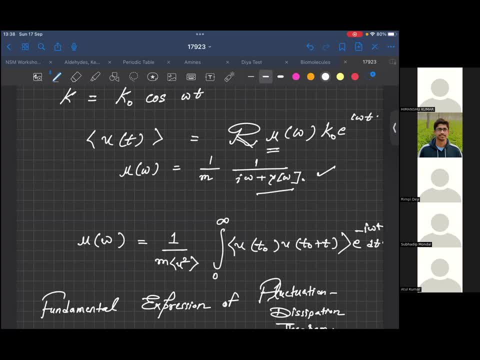 Okay, you can share the paper also. Yeah, I will share it in the group. Yeah, and so basically, this mobility is connected to the susceptibility. So I, yeah and yeah, correlation, spectra part- they will talk about this dissipative part and softy part is related to the position, velocity, articulation, susceptibility, basically in the guy or mix. 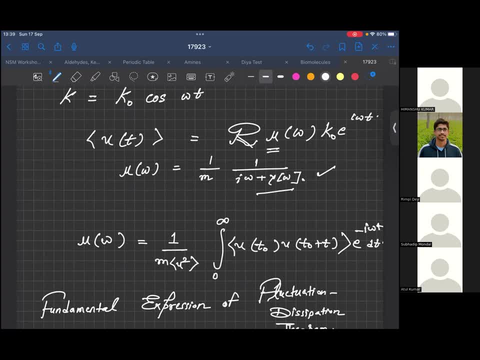 Yeah, And this is not the fluctuation decision theory. Like, okay, you have this fundamental expression right. A fluctuation distribution theorem is like relationship between fluctuation, That means noise And this is going to be a fix. Okay, so relationship between the friction and the noise term is the fluctuation distribution theorem. 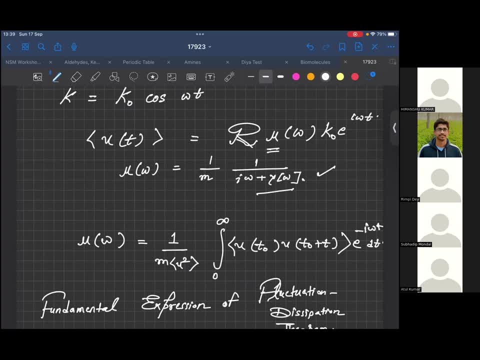 So this is, you can call it, this is mobility or dynamic mobility or susceptibility, You can call it. but Yes, yeah, Yeah, The general expression for fluctuation, distribution theorem, Non Markovian process or generalized engineering equation is different and which is like is the relationship between the gamma as a function of Omega, which is friction, and it is related to the noise part, which is 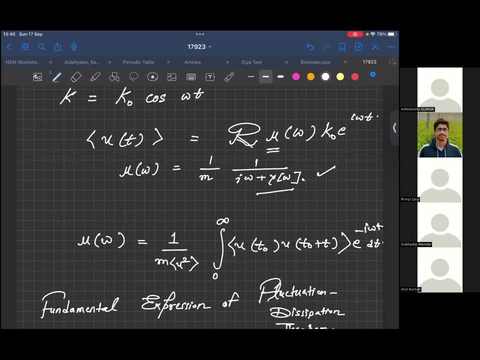 you are in your expression RR of random force. circumstances brought up Mm. hmm, Okay. okay, this is what I wrote from this paper. was written in there that this is a fundamental expression. Yeah, you can derive it from here also. 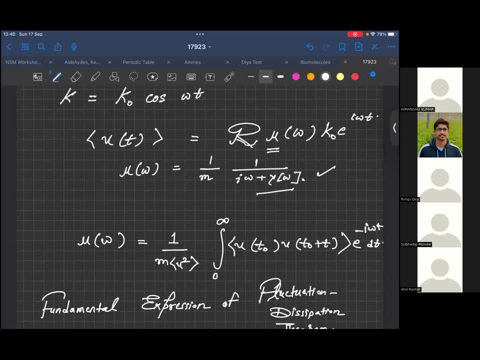 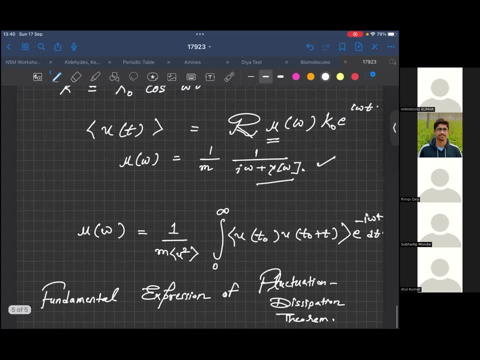 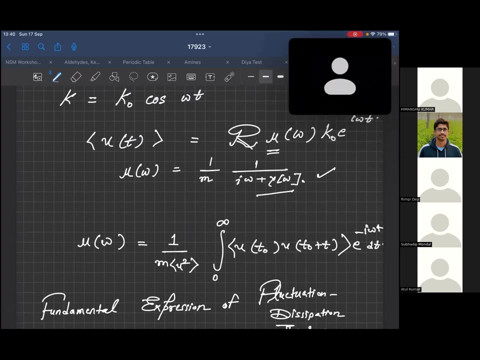 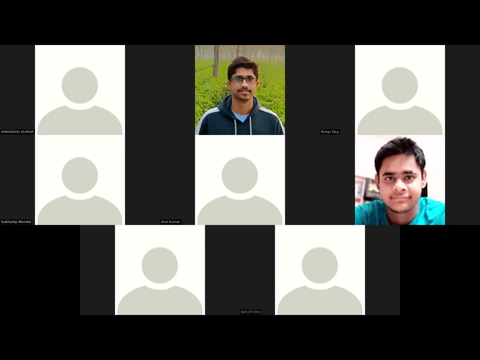 Okay, So yeah, basically I was a little bit wrong, because this is called the first order fluctuation distribution theory, like first fluctuation distribution theorem. Yeah, And the main fluctuation distribution theorem, which is the relationship between the friction and the noise.